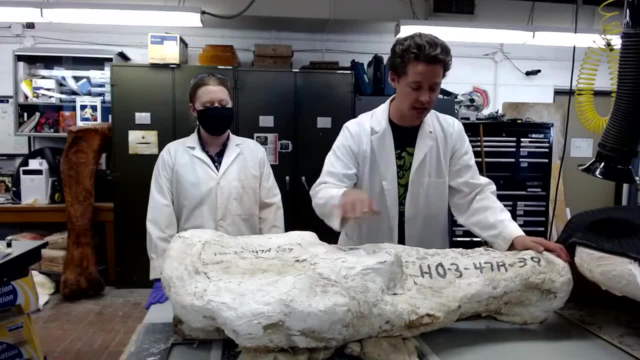 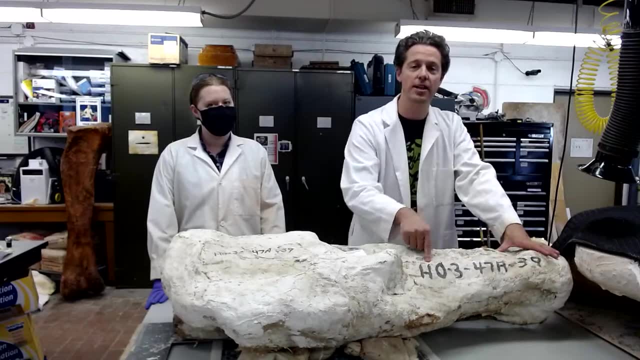 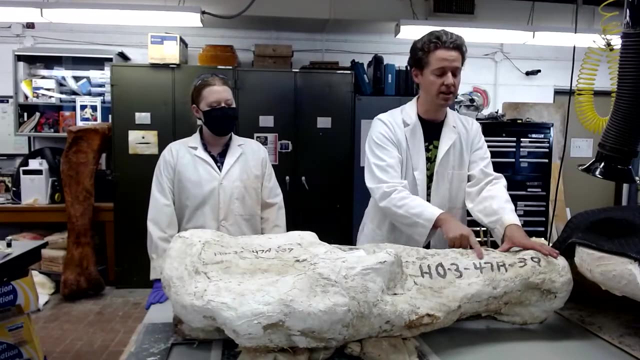 localities in Texas. Now this is our jacket. We have a number here, HO347A39.. This is HO is Howard County, so that's up near Big Spring. It's quarry number three and jacket 47A and it was collected in 1939.. We're not really sure what. 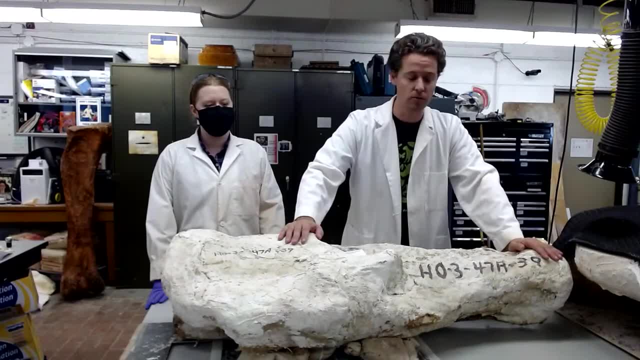 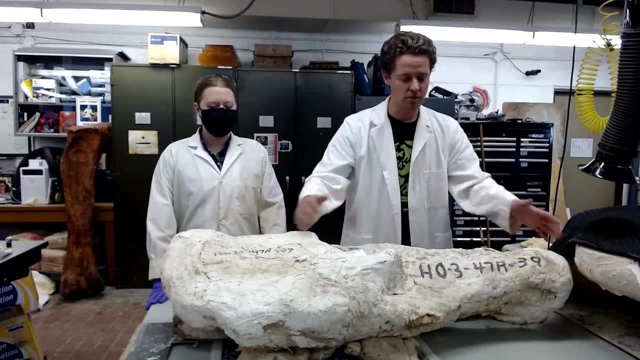 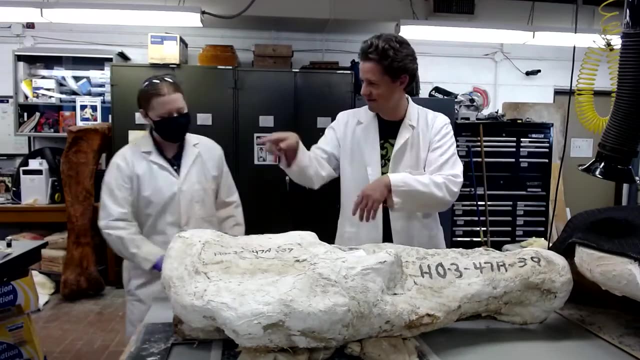 this fossil is. It's really difficult to tell what a specimen is when it's still encompassed within the matrix in the field, but the general shape of it makes me think that it's probably something like a phytosaur. Yes, okay, Hang on a moment. 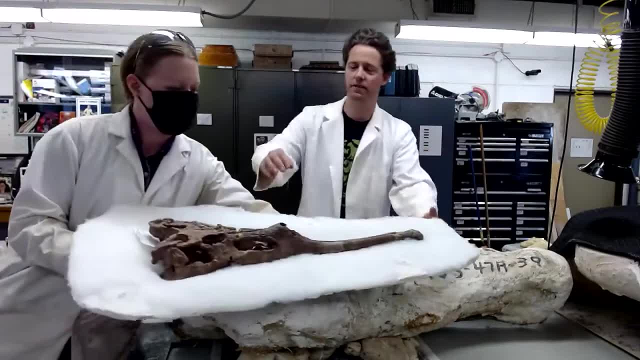 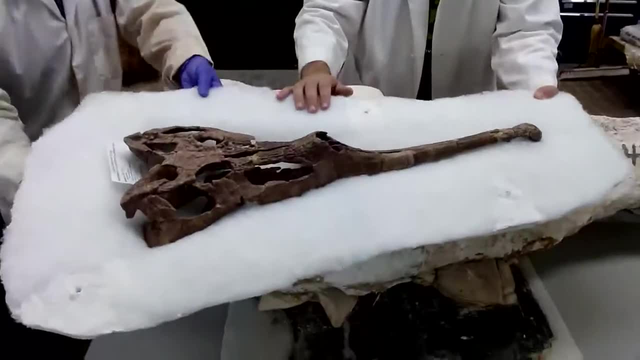 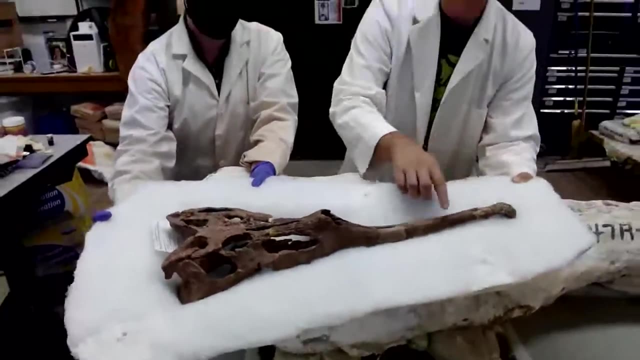 So here's a phytosaur skull. It's roughly the same shape as the jacket. Phytosaurs are crocodile-like animals that are distantly related to crocodiles, and the main difference is: in a crocodile you'd have the nostrils up here, but they're actually retracted to just in front of the eyes on a. 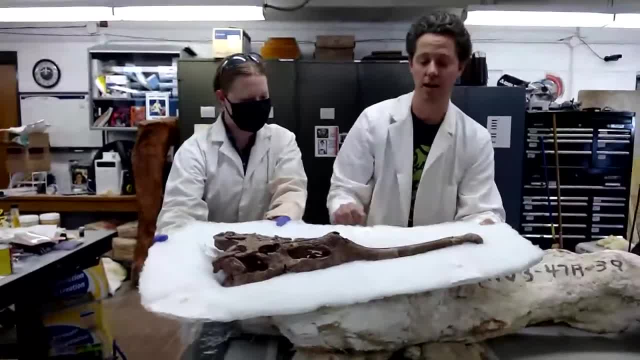 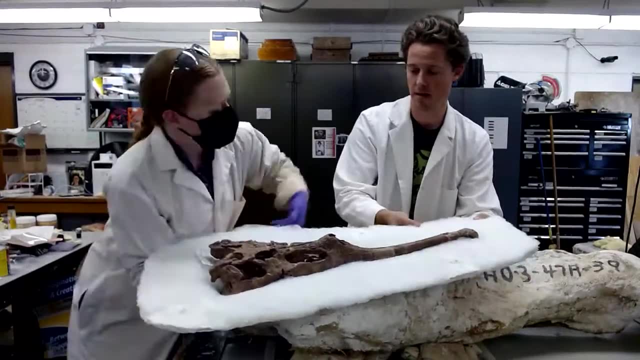 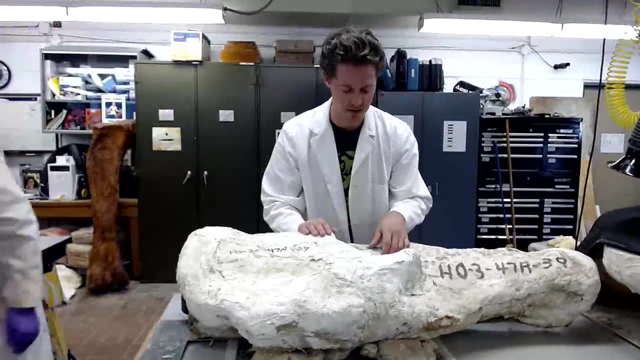 phytosaur, and these are probably some of the most common animals we get during the Triassic in western North America. So we're going to go ahead and open this up. No promises that it is a phytosaur skull. I've had some times. 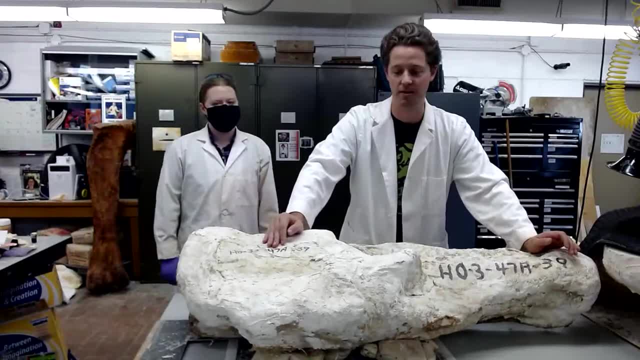 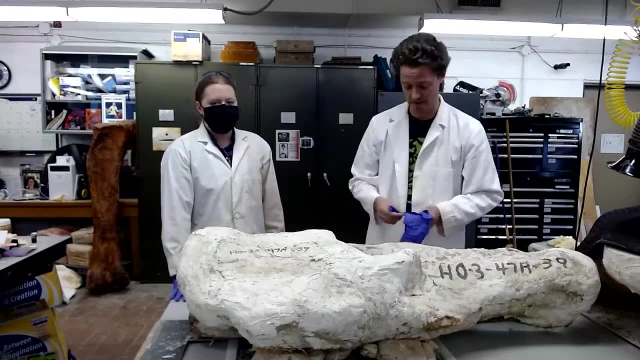 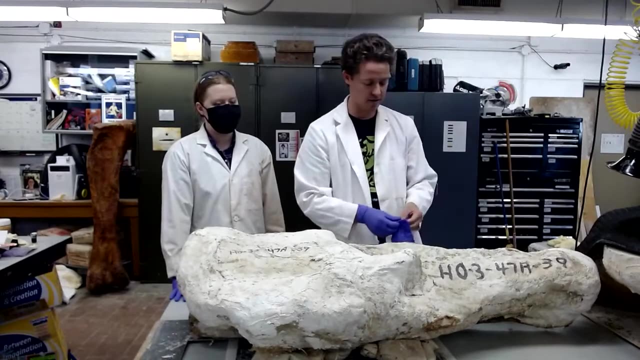 where I've opened up a jacket and found it's not actually part of the Howard County Otis Chalk fossil deposits. but we won't know until we open it up. So I'm going to use a tool to open it up that makes a little bit of noise. It's called a Dremel tool. 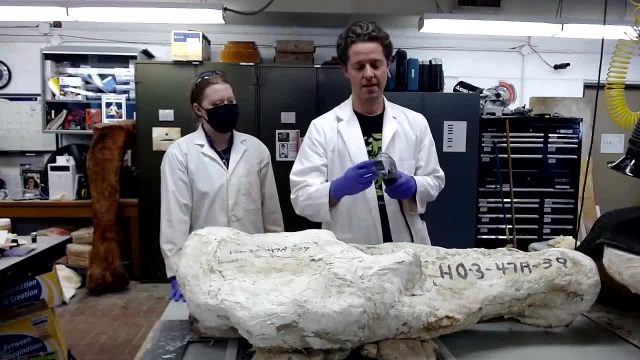 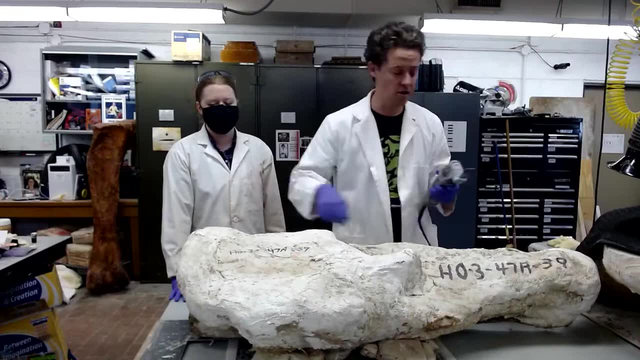 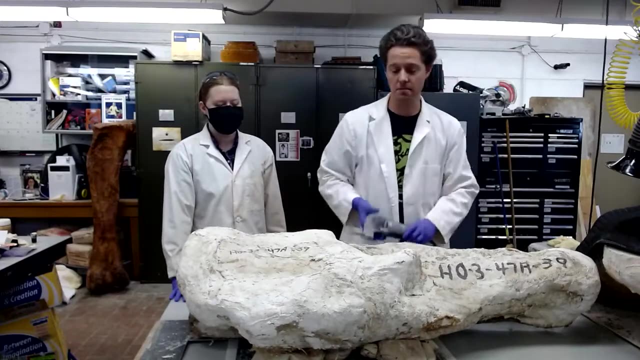 And it's basically a vibrating saw, like a cast cutting saw that I'm going to use to cut away at the plaster and open up the top of it as a lid. I actually already started opening the back side. This is going to make a little bit of noise, so expect it to be a little bit. 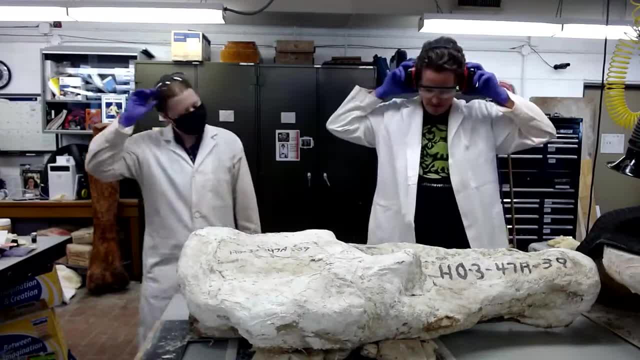 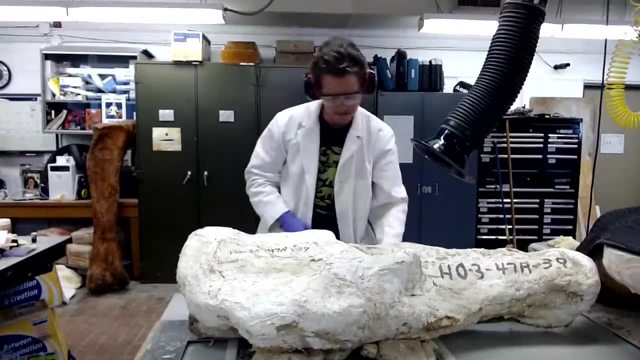 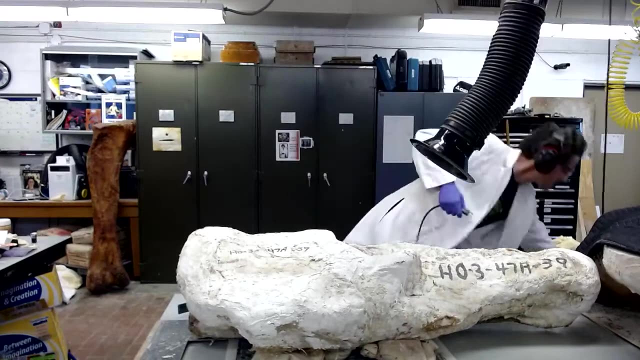 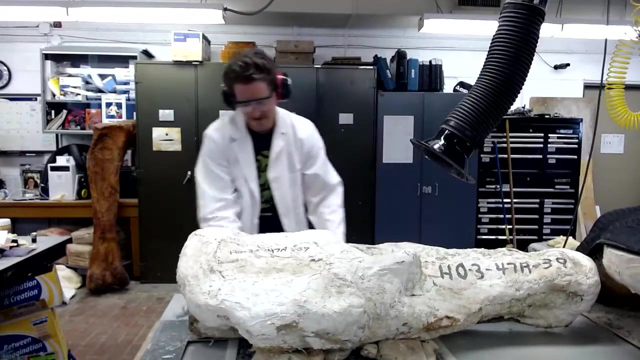 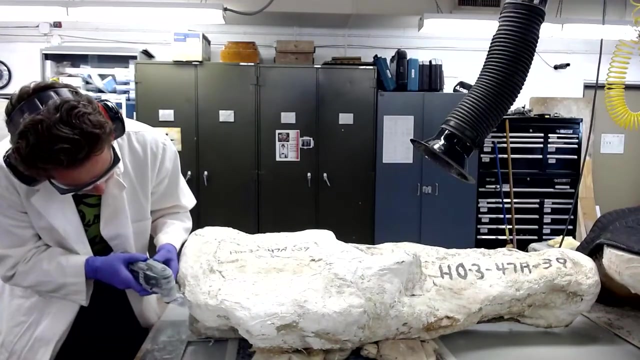 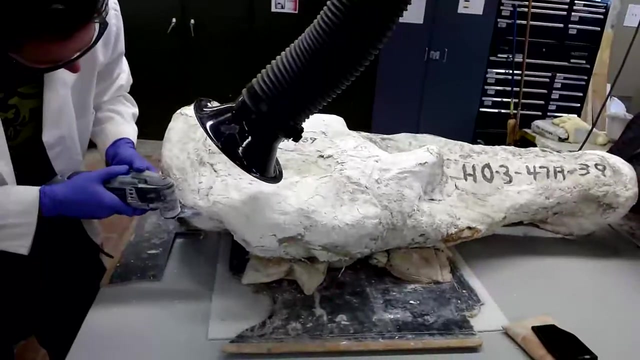 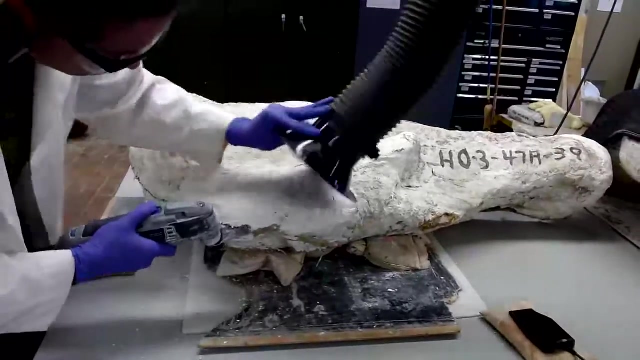 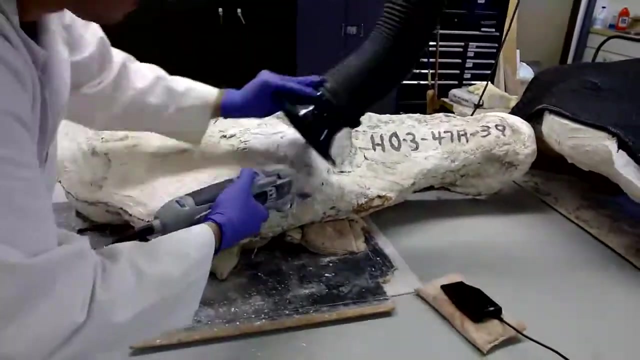 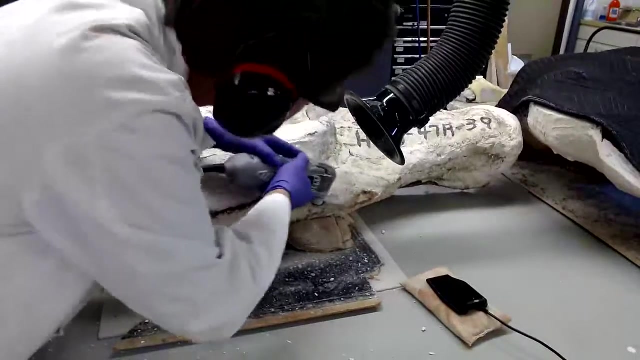 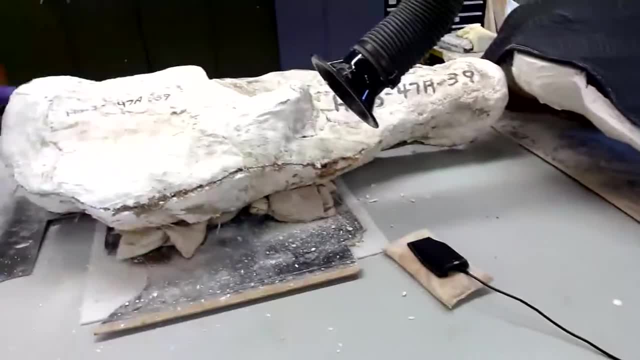 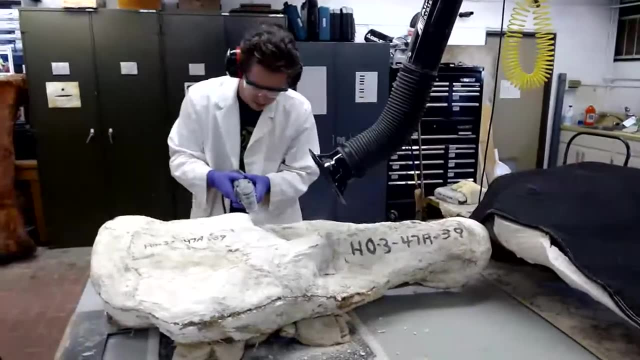 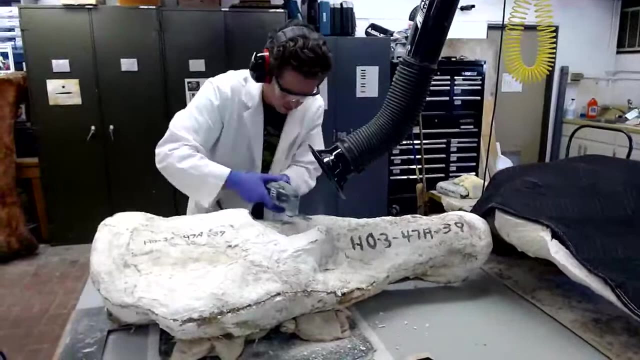 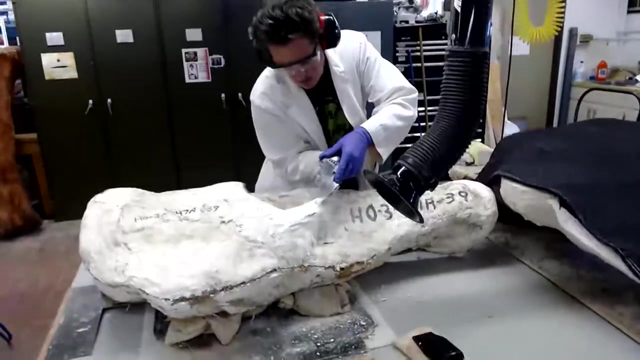 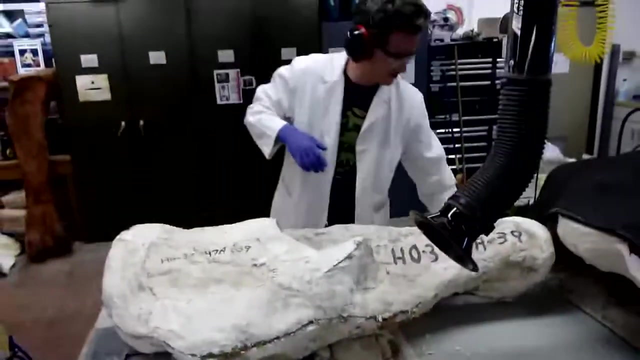 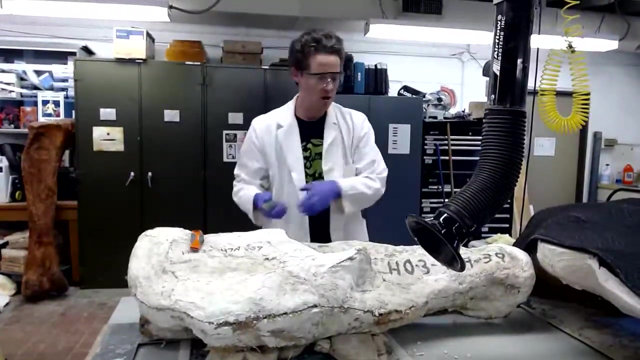 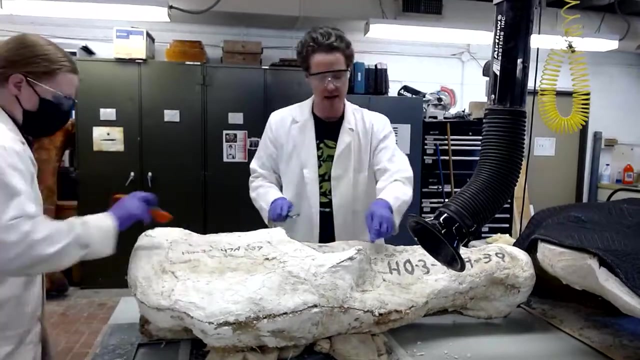 Yeah, Oh, Hum, No, Hum, Hum, Hum. Hopefully that was enough, and now we are going to trim the last little bit open with X-Acto knives to cut the burlap on the inside of the plaster. I made a few extra incisions up here just to kind of help make sure that the jacket 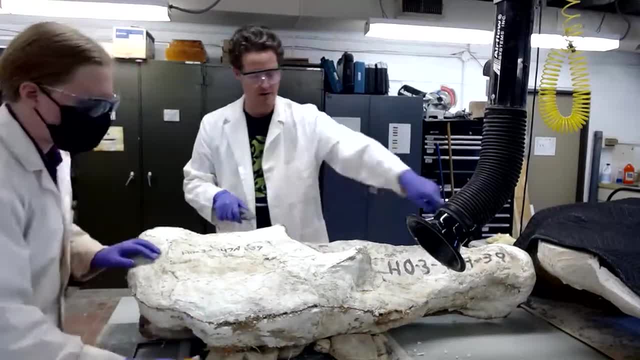 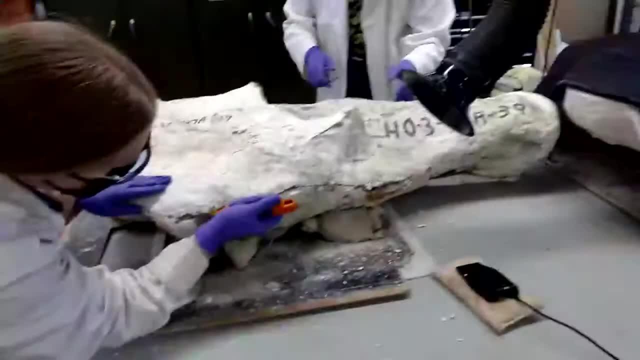 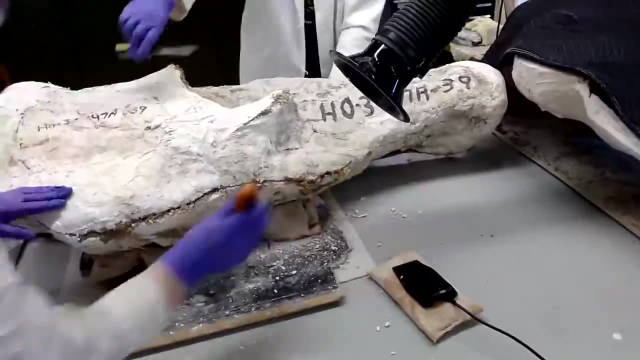 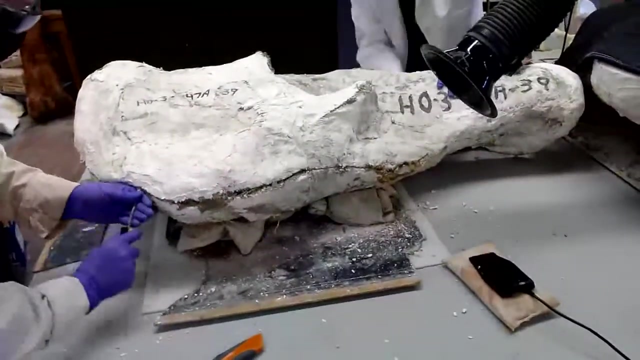 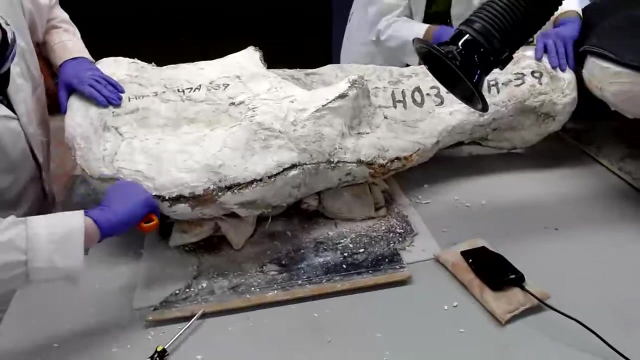 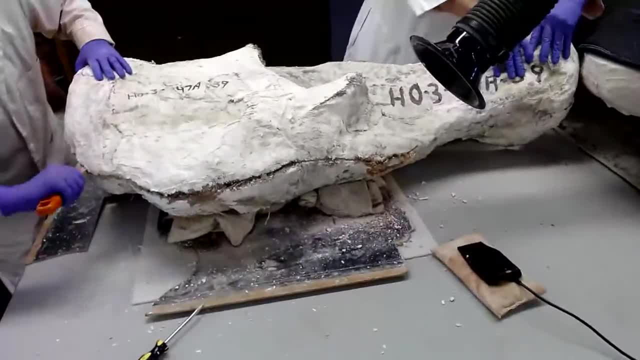 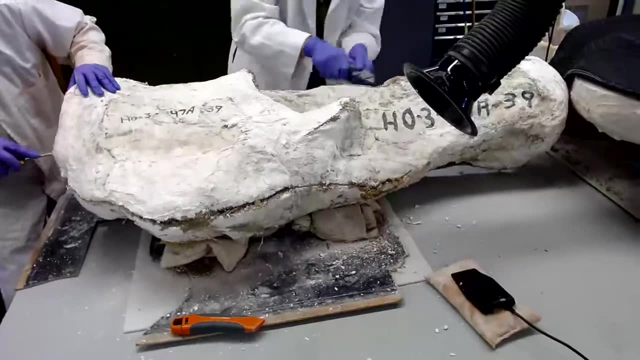 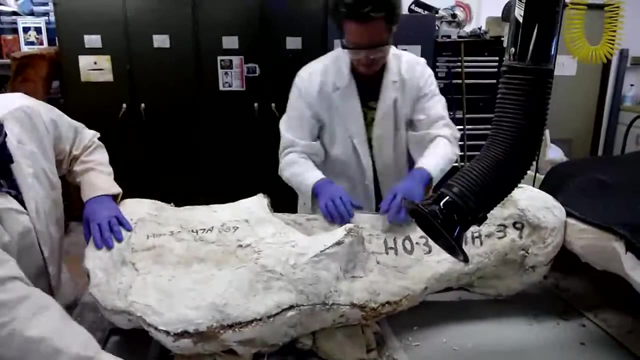 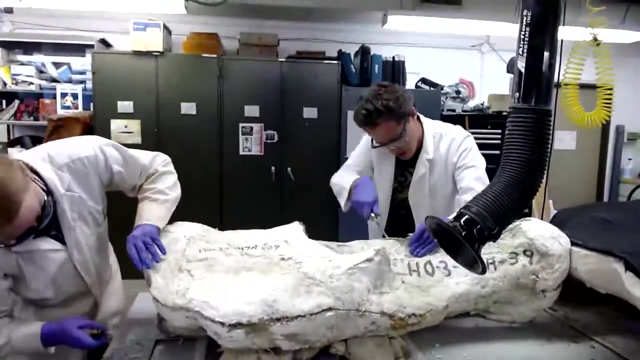 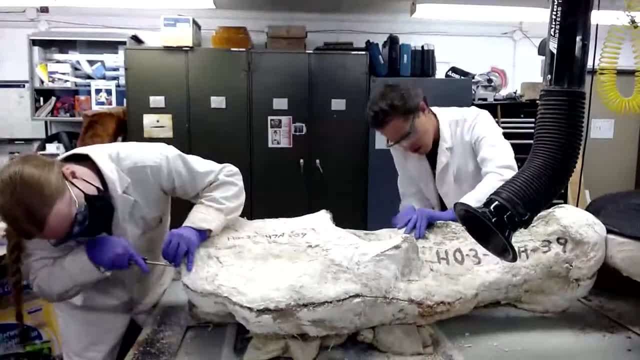 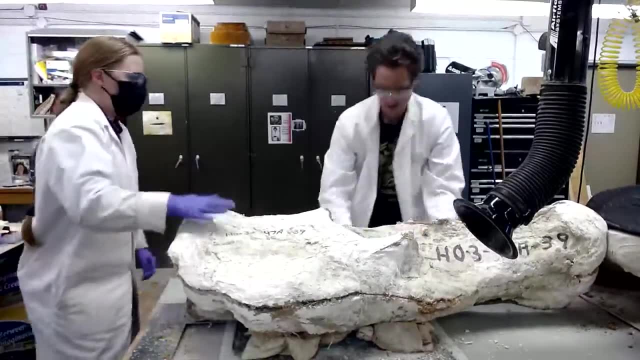 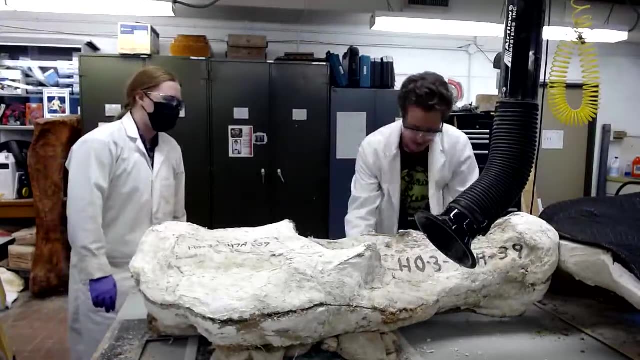 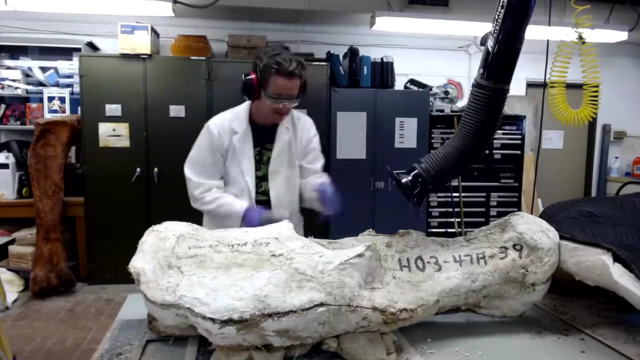 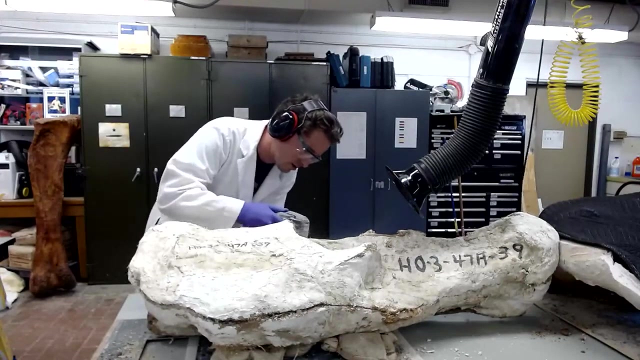 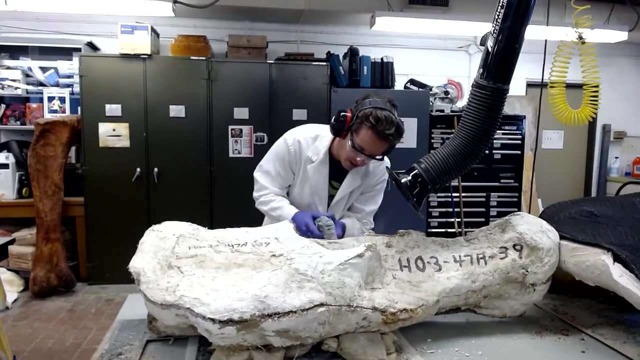 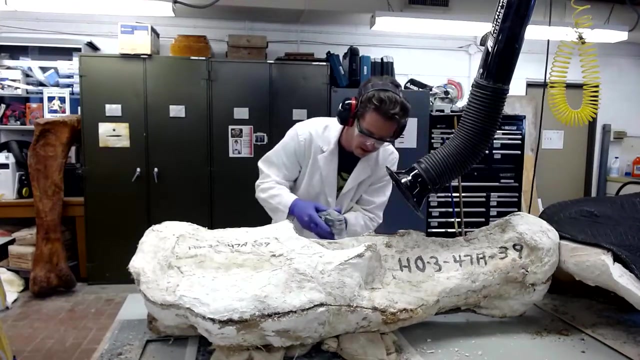 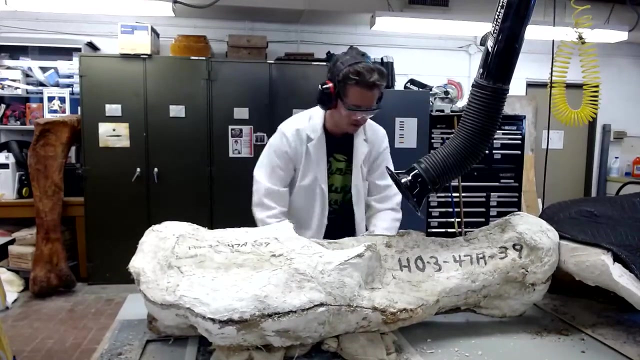 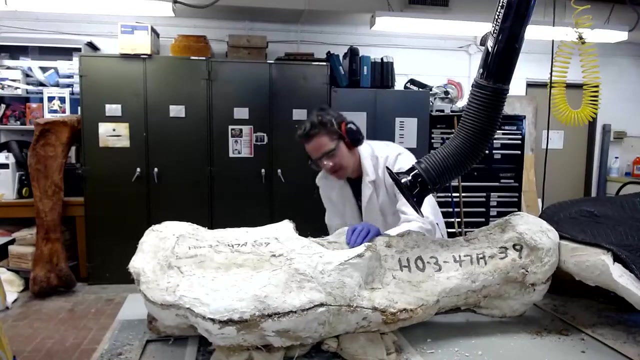 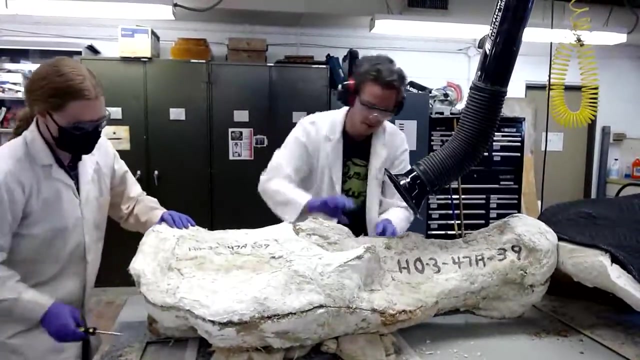 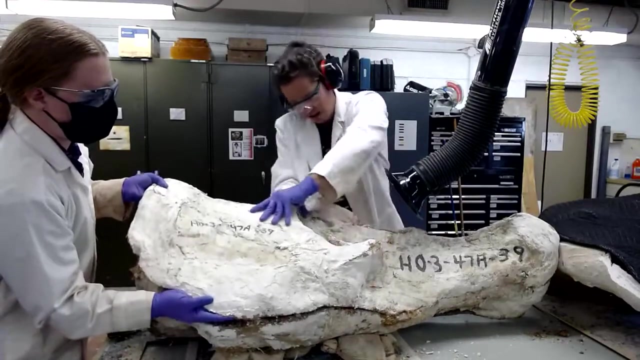 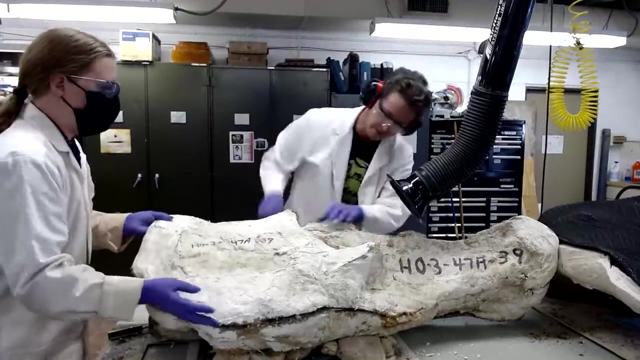 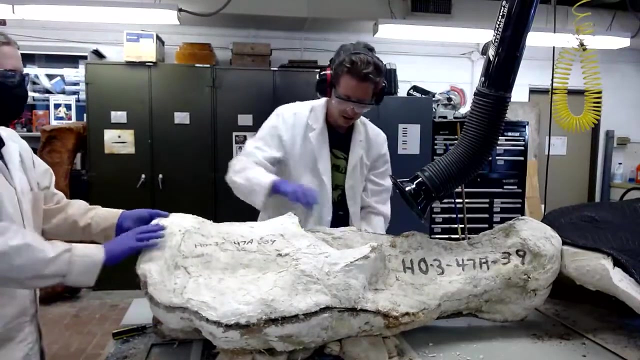 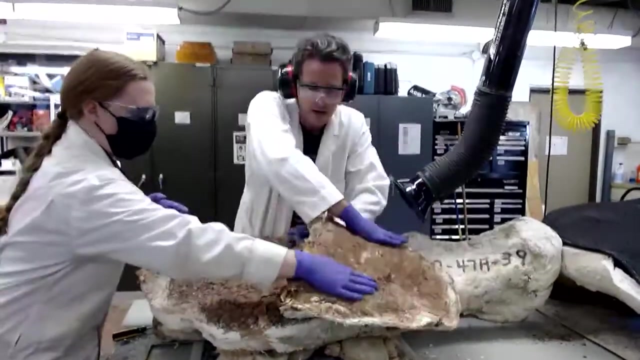 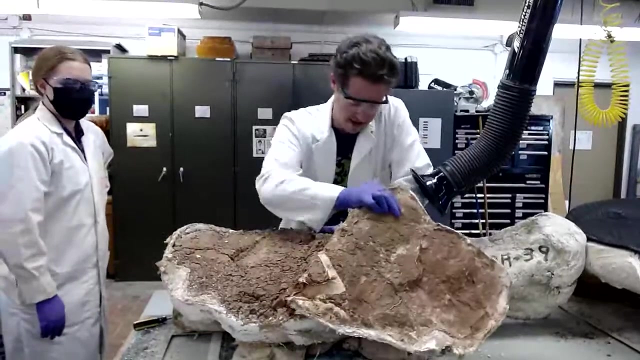 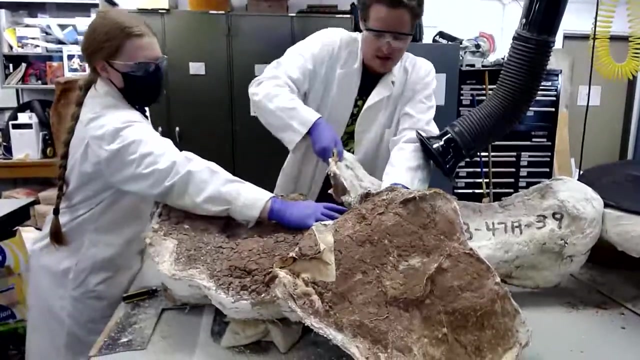 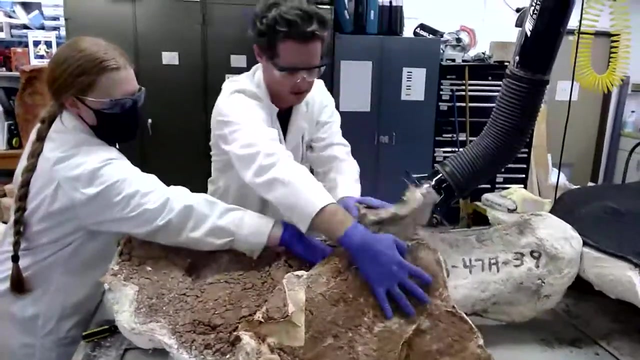 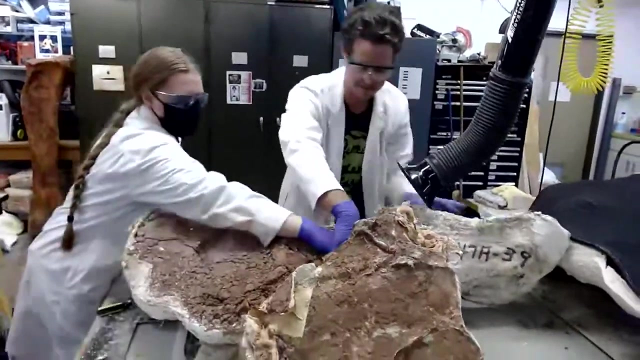 Here. Okay, Yes, Okay, Okay, Okay, Okay, Okay Again, burn the ol. if youủ Got your, I need to cut and separate here. Well, I guess we're not getting coal this year. There we go. We've got a lot of loose matrix right up here. 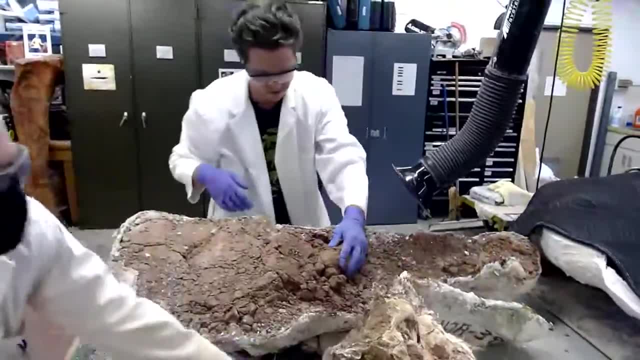 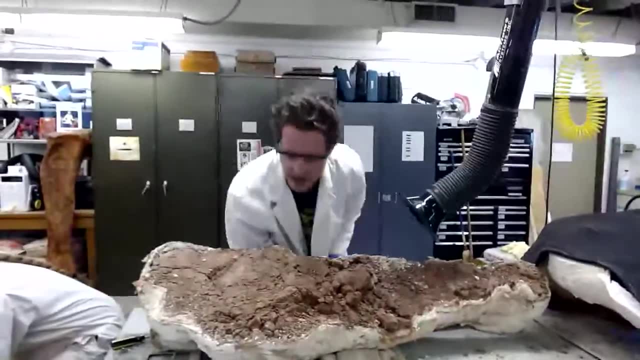 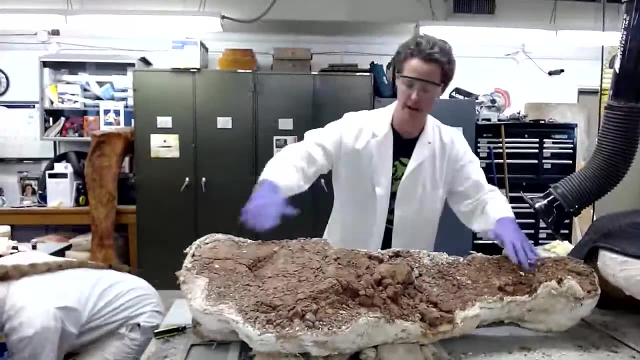 Let me go ahead and just take that lid off. Well, the good news is I'm not seeing any bone right now, Maybe a little bit right here, So we're just going to go ahead now and start cleaning up a lot of this loose rock. 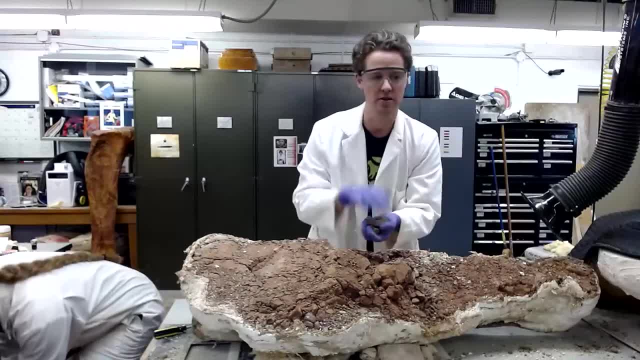 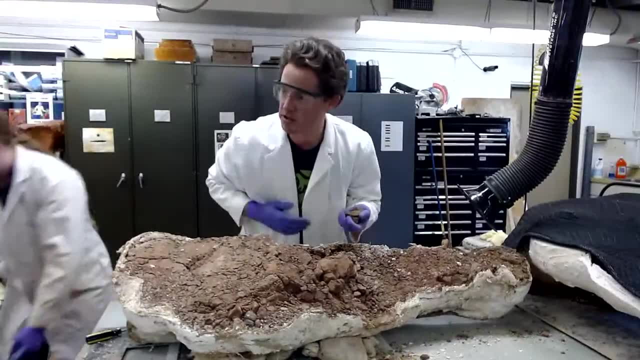 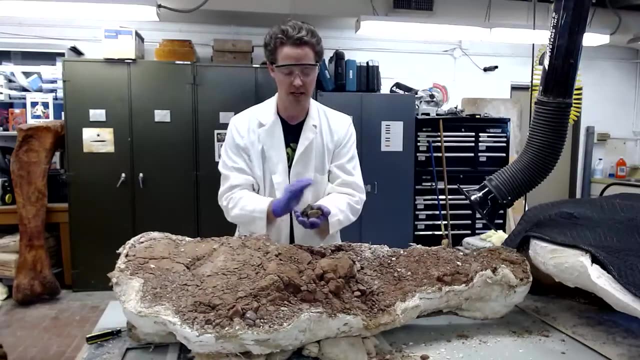 Okay, It appears that this is the rock that was underneath the fossil when it was excavated. What happened to our bucket? We had a bucket. We usually keep – we save a lot of this matrix so that we can screen, wash it and hopefully find either fragments that we missed while we were preparing the specimen. 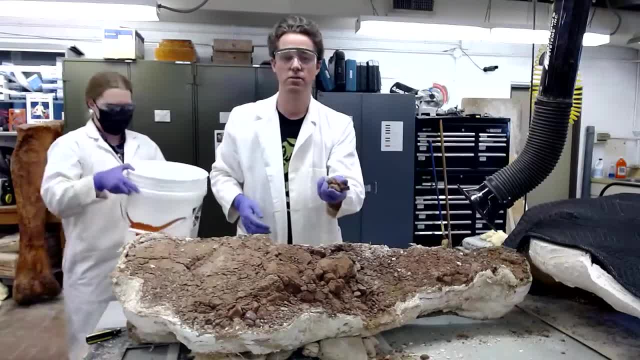 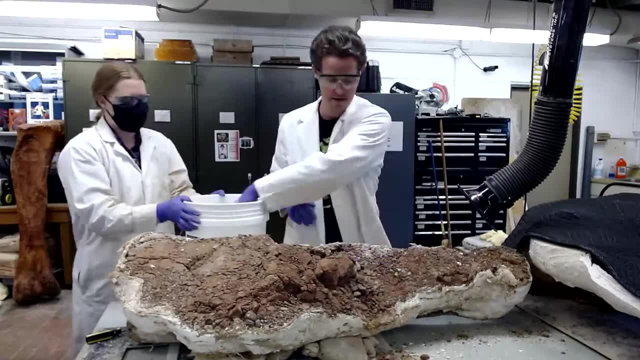 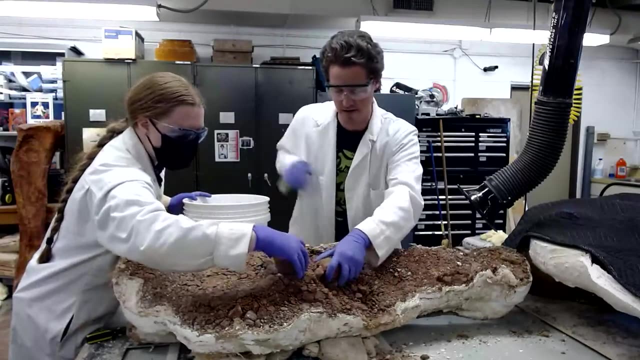 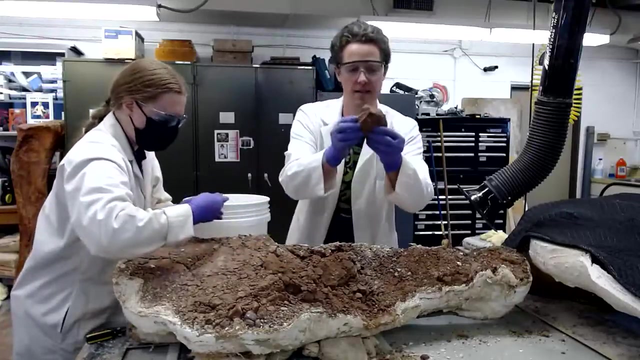 or sometimes we get microvertebrates, things like fish teeth and fish scales and lizard teeth, Lizer jaws and frogs, stuff like that. Just carefully look at each piece and make sure there's no bone as we go. Most of this is just a silt stone or a mud stone with little green clay clasps in it. 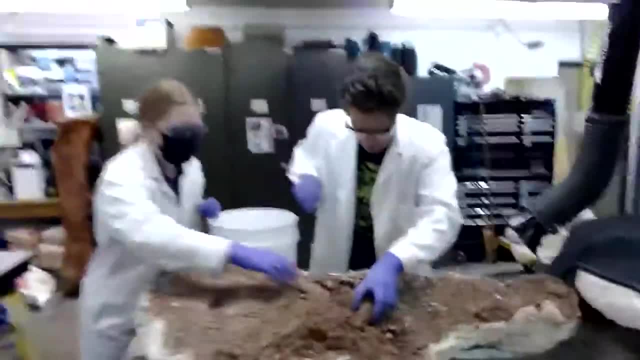 Okay, Let me try and see if I can figure out what it is. It's a little piece of felt stone. It's a little piece of felt stone. Okay, I can't believe. I can't believe it's been so long. 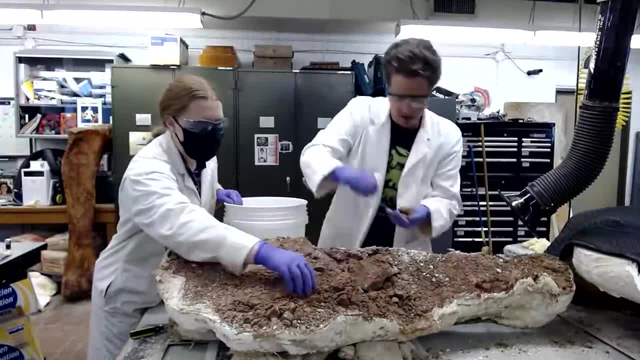 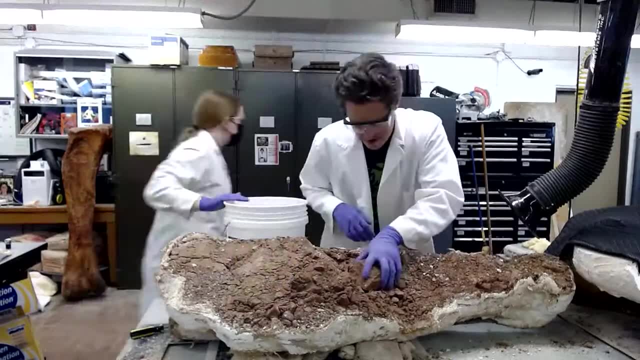 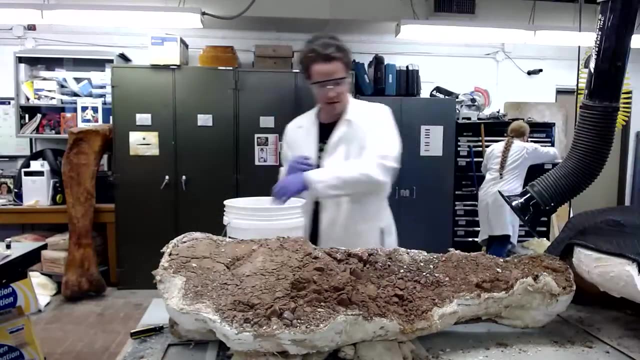 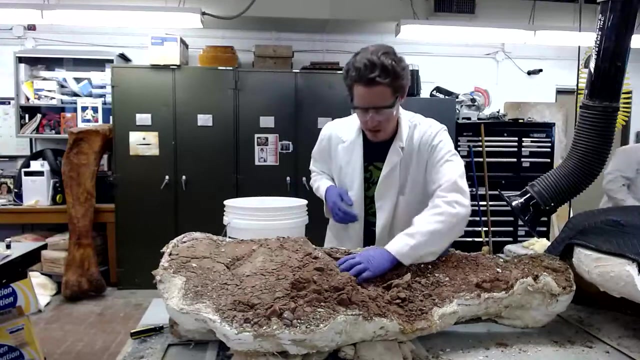 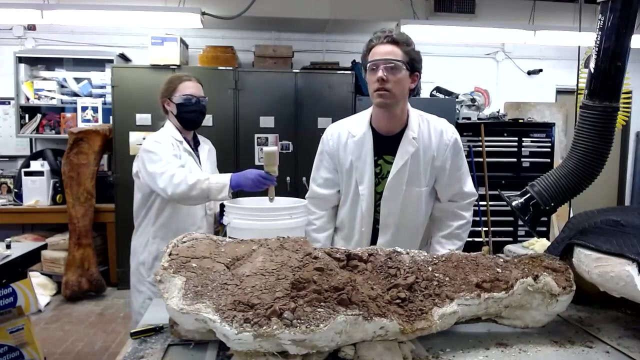 I could never have guessed this, but it's so much work I don't know. Congratulations, we actually got a question. do you guys find answering it? yes, what's your question? yep, can you guys tell us a bit about the geology of the locality? and that's a question from renee. 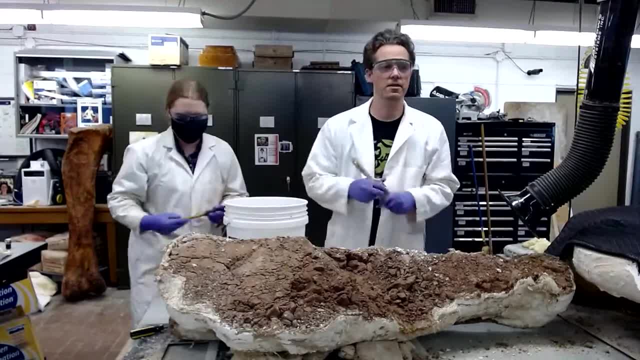 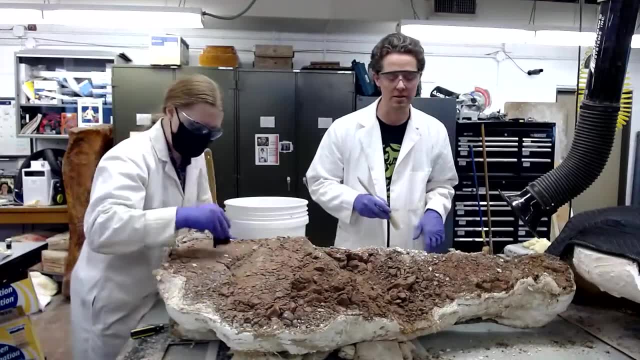 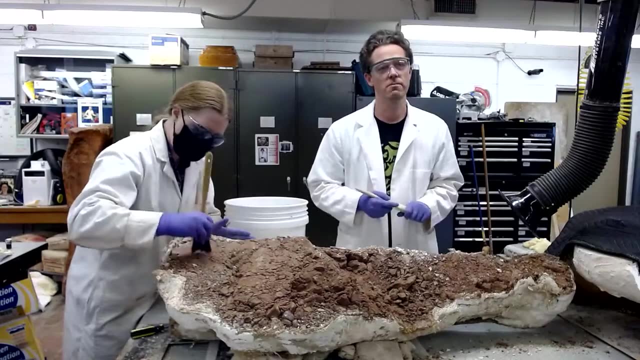 okay, um, i don't know a lot about the geology from the locality because no one's been out to the locality since it was collected in the 1930s, but the locality is upper triassic in age, out near big spring, and it's mostly composed of mud stones and silts- silt stones. 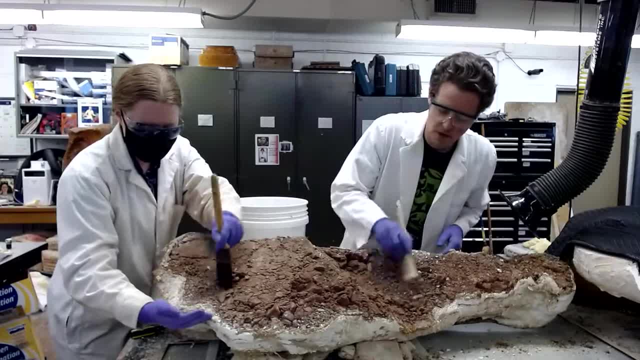 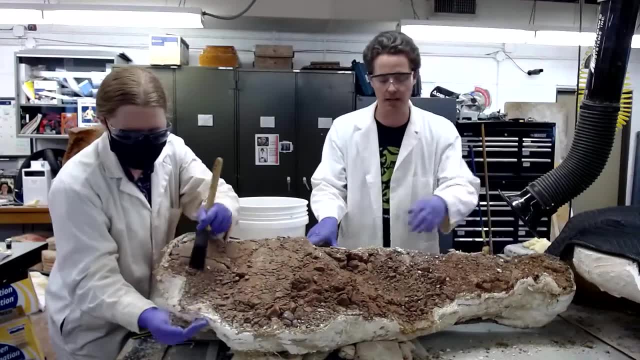 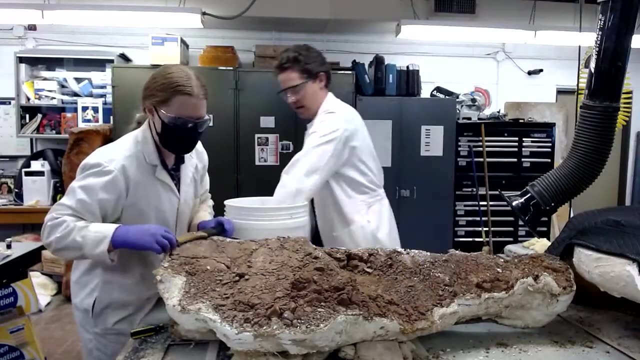 um. overall, the locality has produced mostly vertebrate fossils, so there are things like phytosaurs and aedosaurs. there are a handful of dinosaurs from the locality and every time we open up a new one of these blocks, since we don't know what's inside. 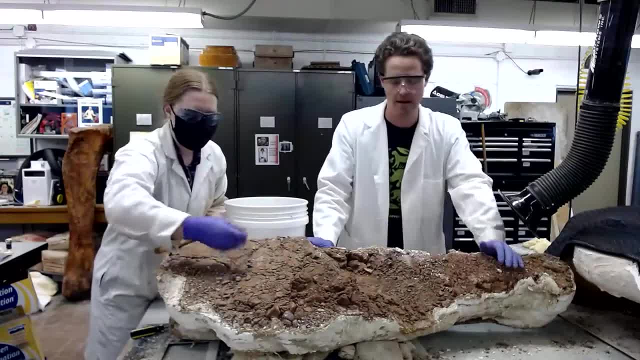 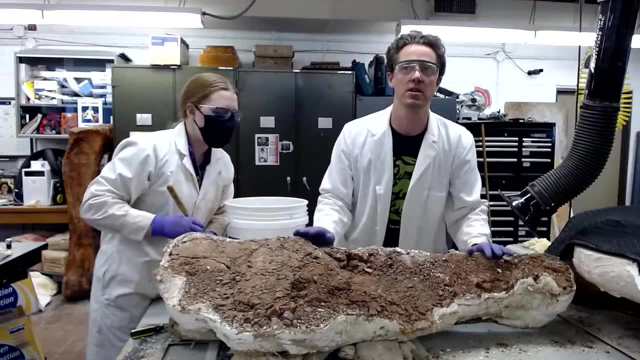 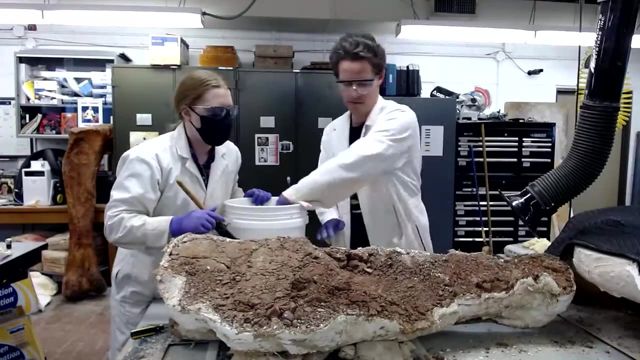 there's always a possibility that we might get some new animals, so it's triassic in age. i think that would put the locality in age somewhere between uh 310 and 330 million years old, so it looks like you've exposed the bone a little bit right here. yeah, there is a bone right there. 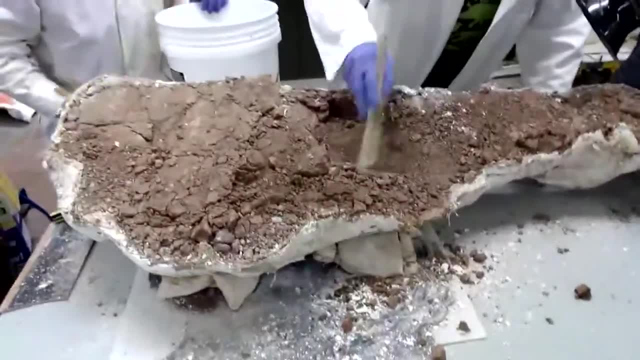 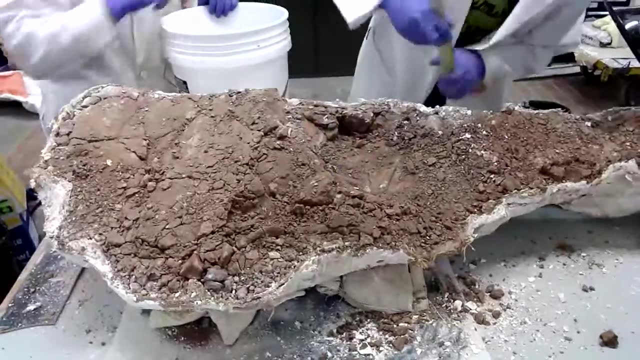 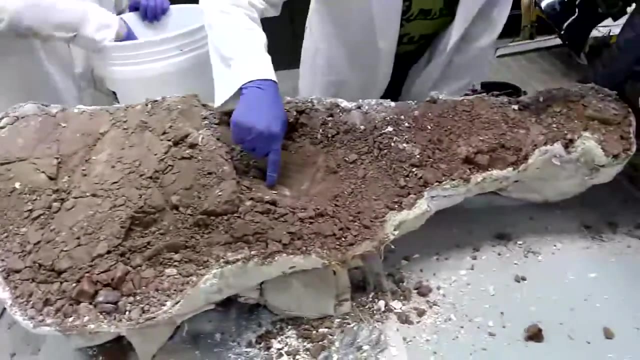 and there's another bone right here. so there's something right here real thin, and another piece here and it's interesting because it it's not something i'd expect to see in a dinosaur skull and it seems like it's almost like a rib-like object and the two halves. 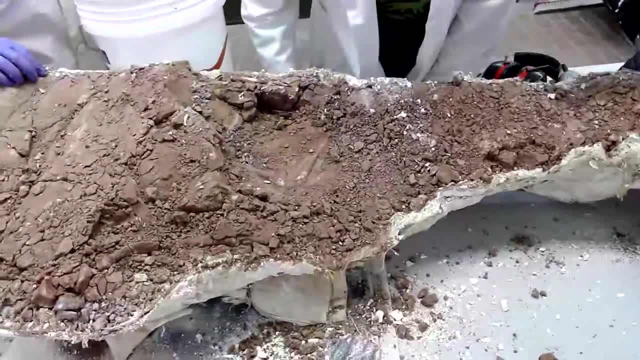 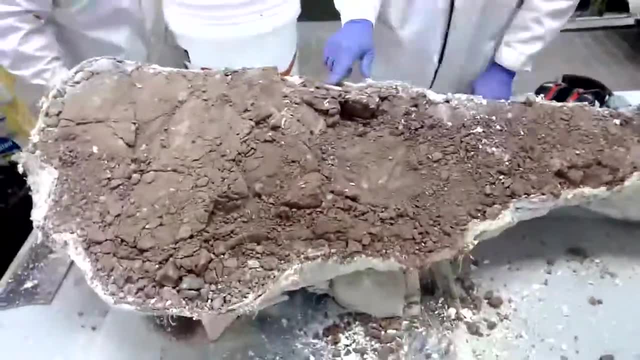 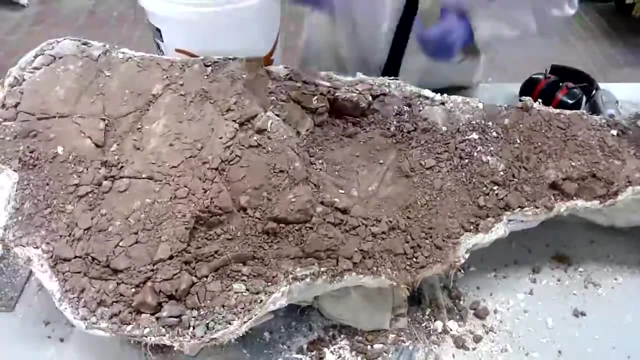 combine and they have a 90 degree turn, which is interesting. there's also a little bit of bone right here, exposed more of it right? i think this is also bone. all this stuff that's kind of whitish is bone and there's a little bit of bone. 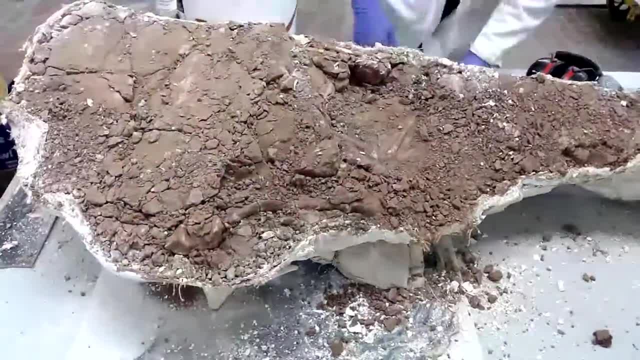 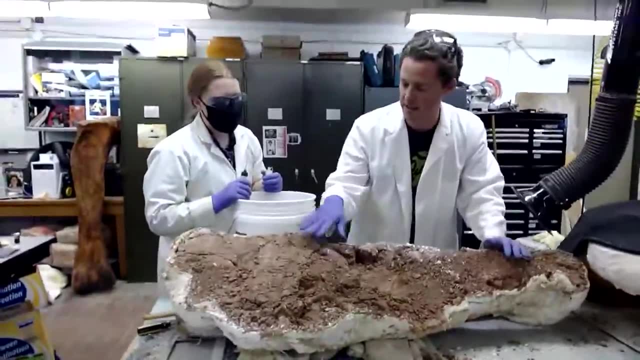 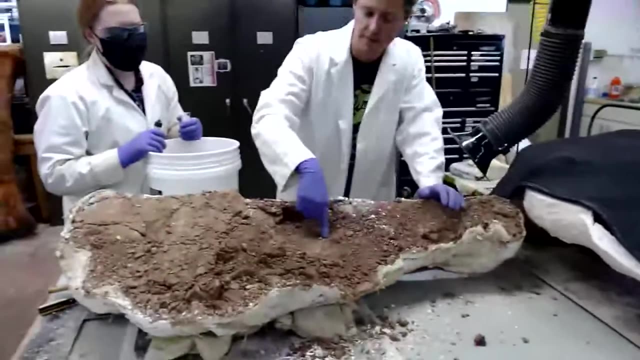 right here. i know it's hard to tell on the video feed generally what i'm seeing right now. the matrix is a lighter color than the bone. the bone has an ironstone concretion over it and it's a little bit more of a brick red color. 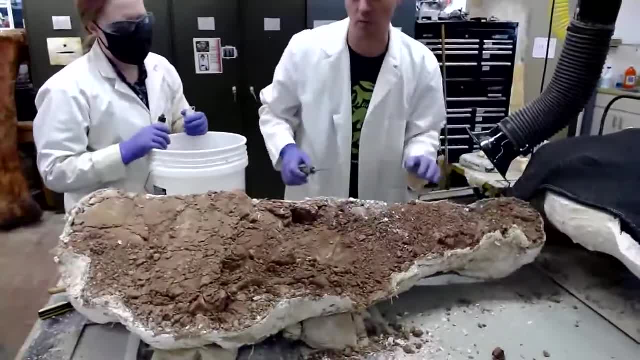 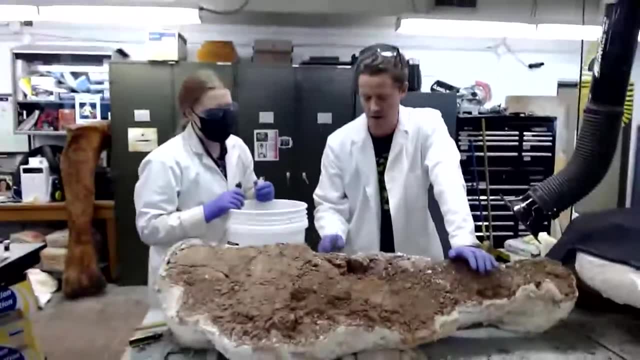 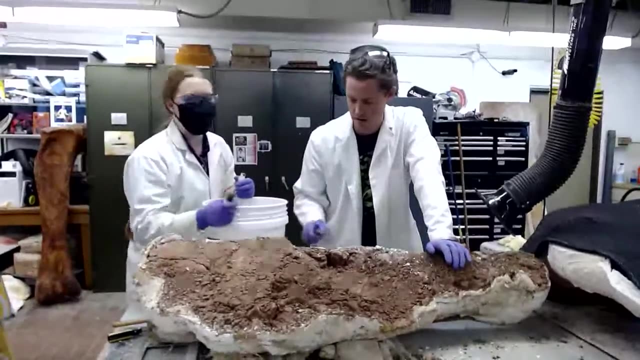 and one of the things that i figured out early on was if you tap it with something metal, you can kind of tell the difference. so here's bone and there's a little bit different. there you go with the matrix. yeah, this sounds a bit more hollow. yeah, more hollow or dull. 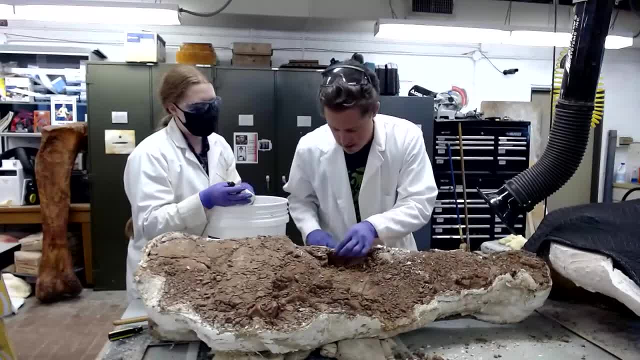 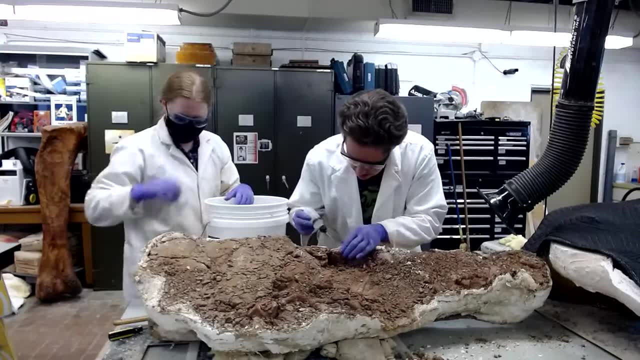 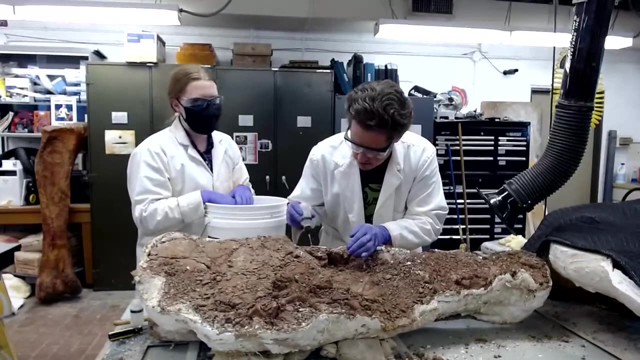 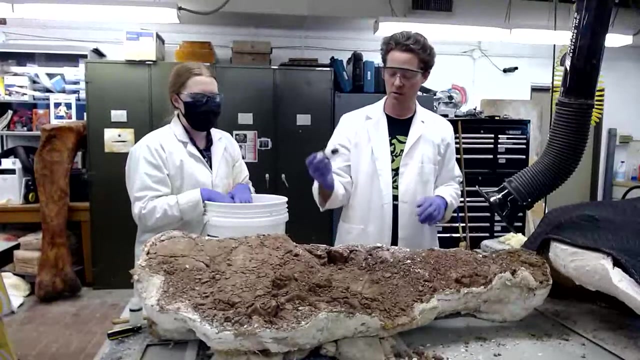 consolidate, yeah something just in case. i know some of it's a little bit mobile, so we add a glue called b72. it's a paraloid b72. it's basically. i always think of it as like a plastic that dissolves in acetone and we drip this into the cracks and as the acetone evaporates away, it leaves that. 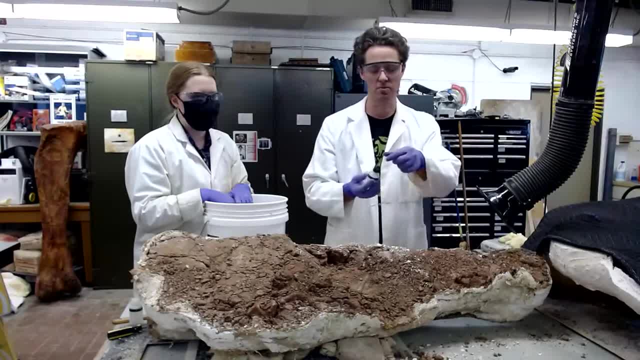 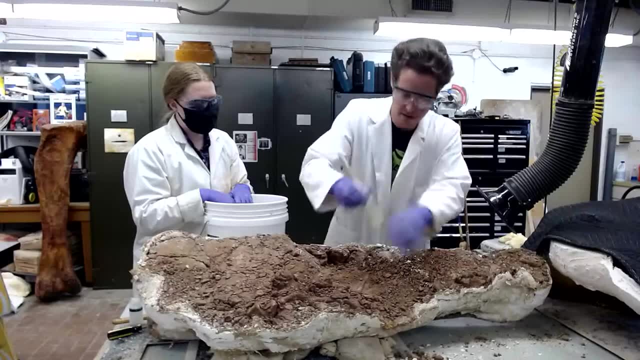 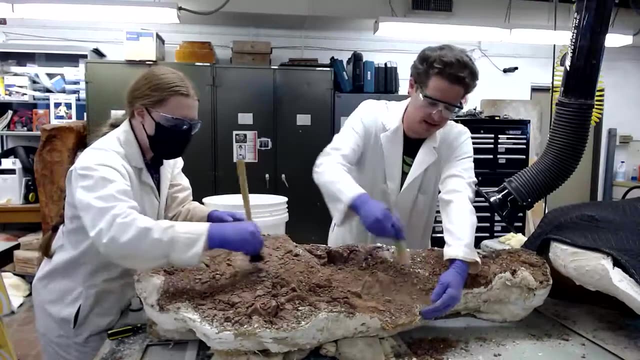 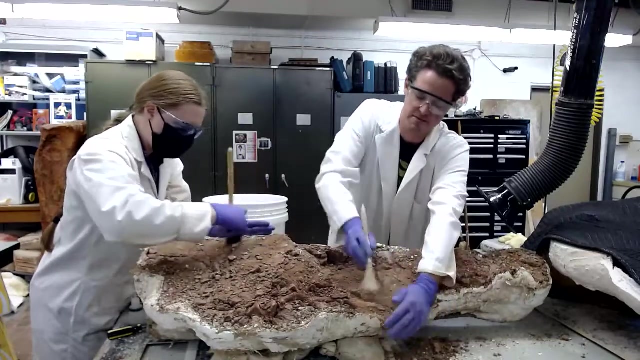 plastic as a hardener and the nice thing is that's reversible. we can add acetone again later on. reverse that glue. i was kind of hoping that we would be looking at the top of the phytosaur skull and it would be easily identifiable, but that doesn't always happen. 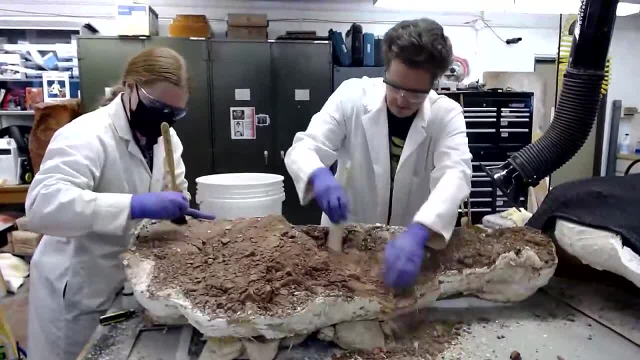 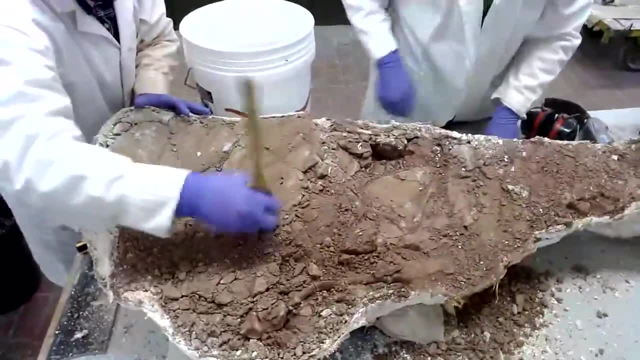 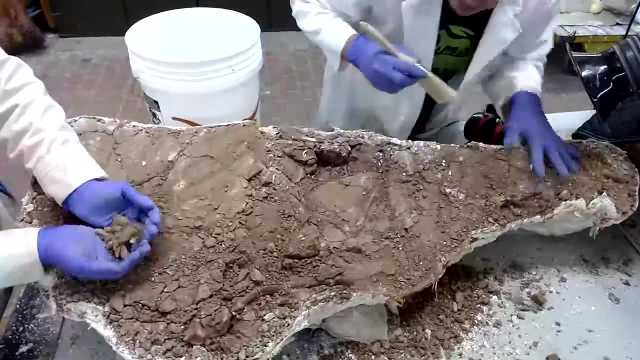 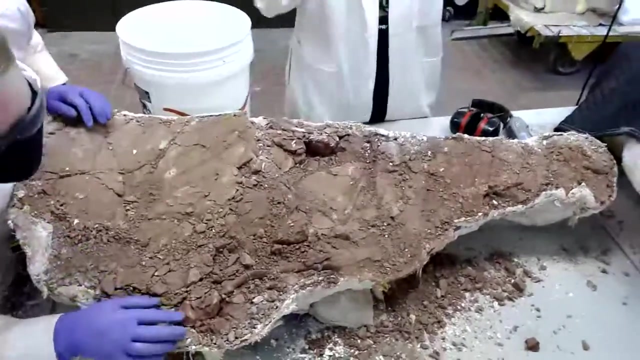 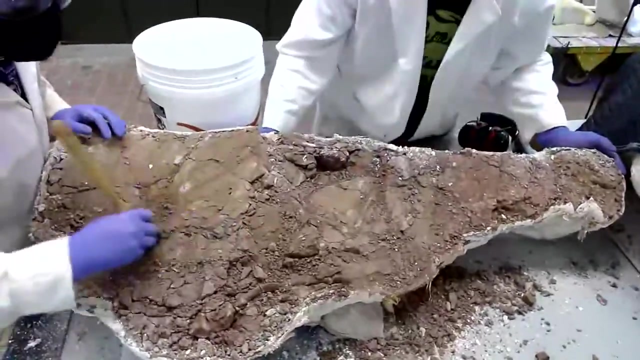 excuse me. we have a question, um, whether this could be a limb bone or not. is that, is that possible? do you see anything could be inside this? there could be limb bones, like that's probably some kind of rib, and i have this. oh hey, check this out right here. 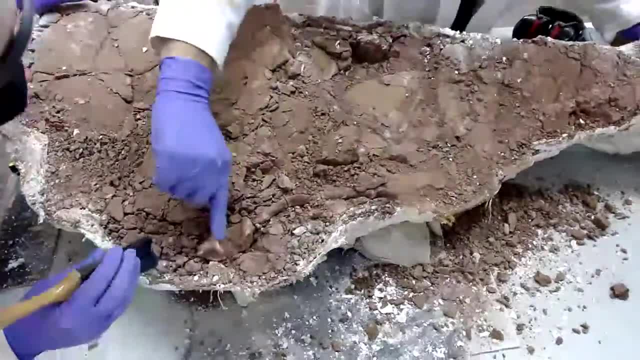 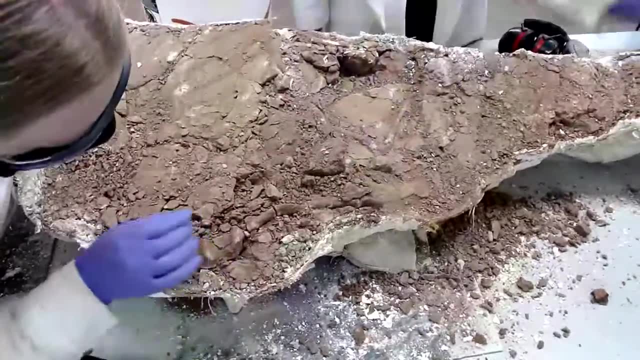 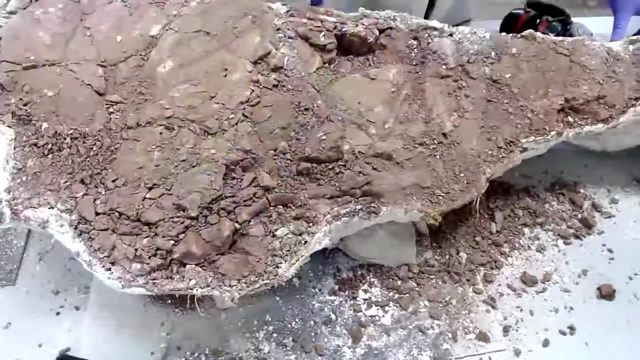 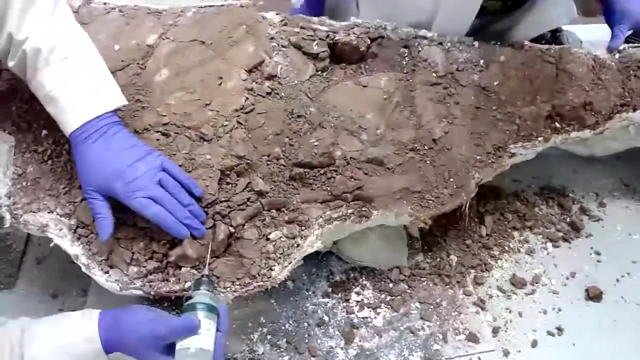 so this is like a socket here, like a joint. so this object right here, uh, the two things i can think of that this could be is: this could either be the socket where the mandible fits into the jaw, so if the skull is upside down, or we could be looking at a scapula like one of the shoulder blades. 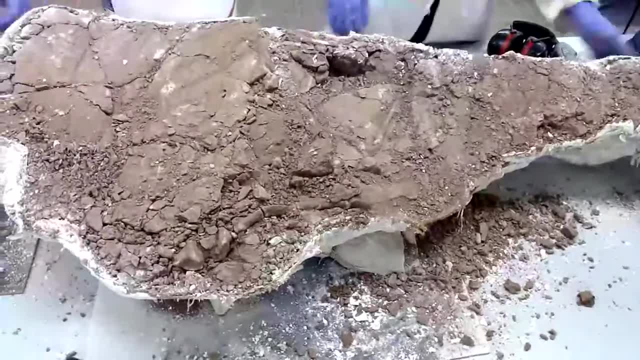 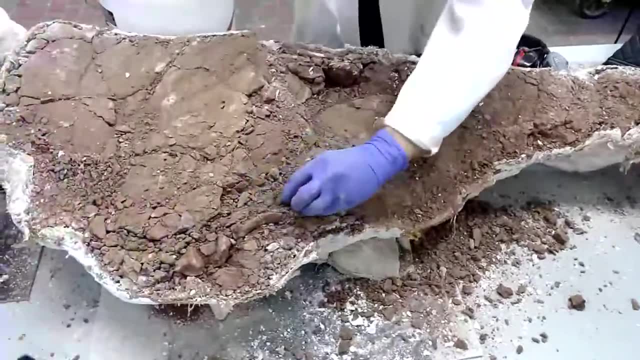 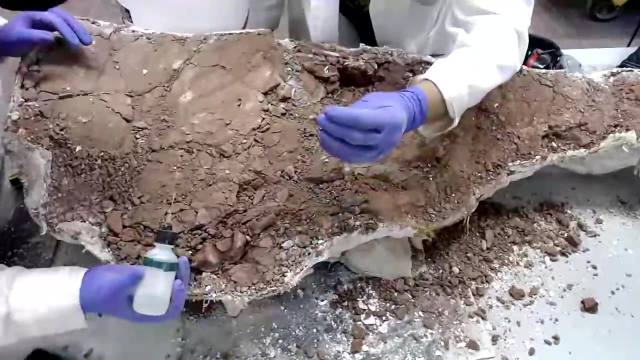 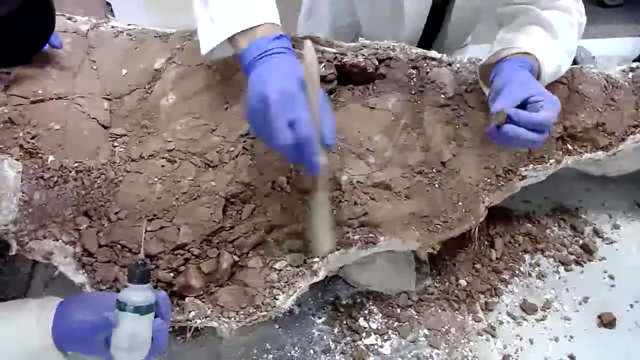 just to make sure it stays. yes, yes, um, hmm, that's loose right there. actually i can. i'm gonna brush away right here before we glue that and see what the shape of this bone is. well, it's not enough to say whether it's part of the jaw or part of the 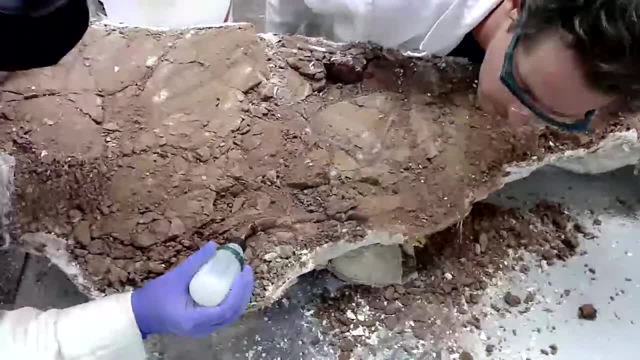 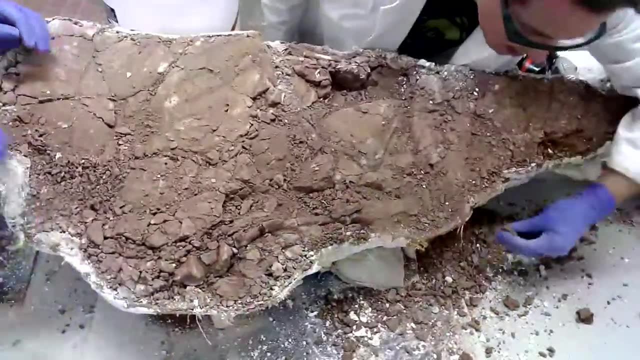 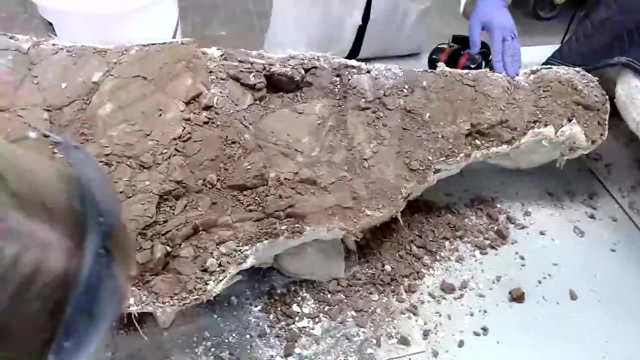 part of a scapula and it appears i brushed away a piece of bone, but we'll find that when we screen wash it. it's probably sitting right there. maybe, if i i'm going to try cleaning here in the hope that maybe i'll expose the underside of the 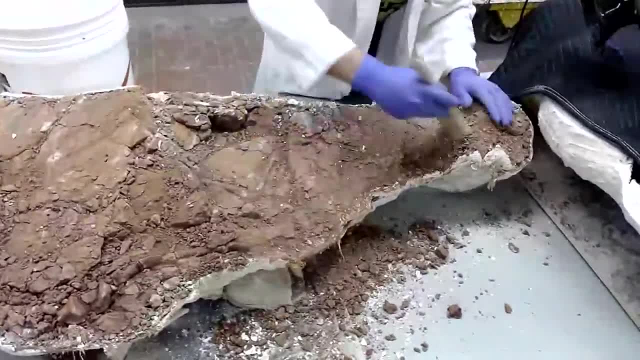 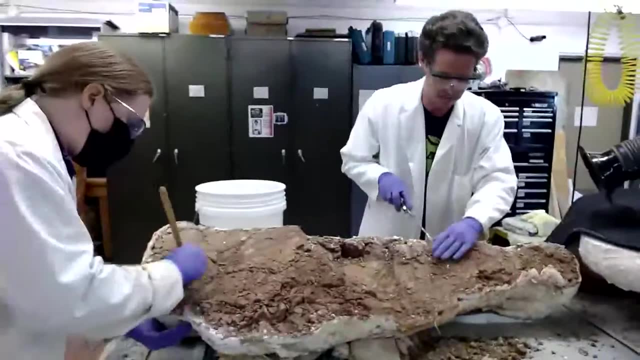 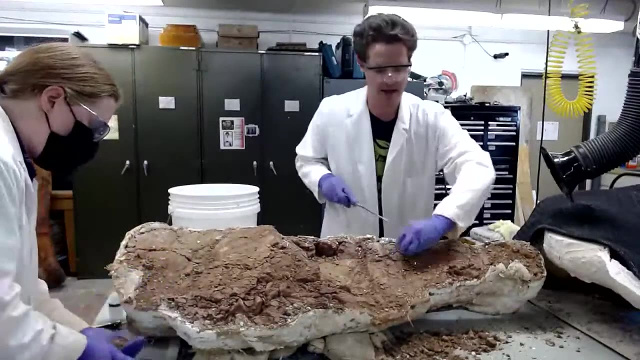 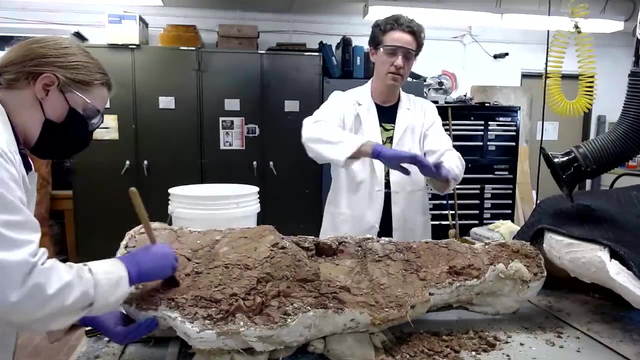 jaw, but yes, we could easily have a limb bone mixed in with this block. i've had a couple of specimens over the years that a couple of these otis chalk blocks that i opened up and immediately right on the top there was a articulated arm and a articulated foot sitting right on the surface. 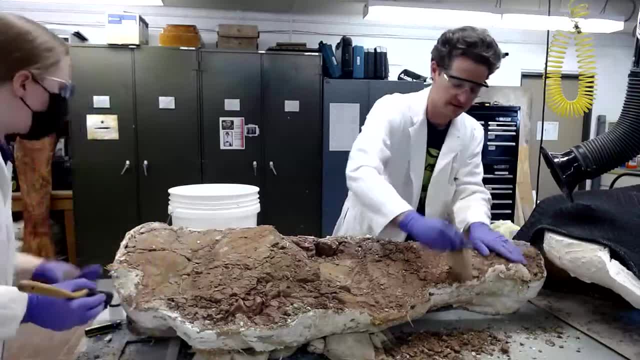 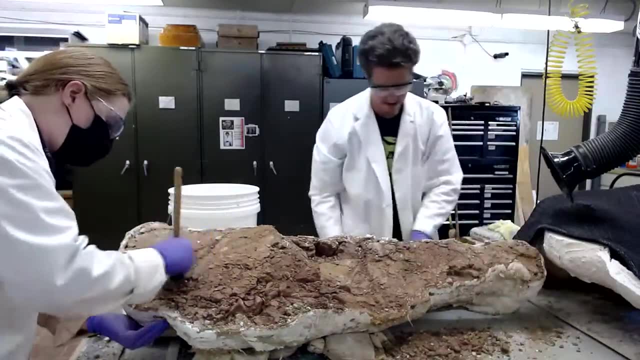 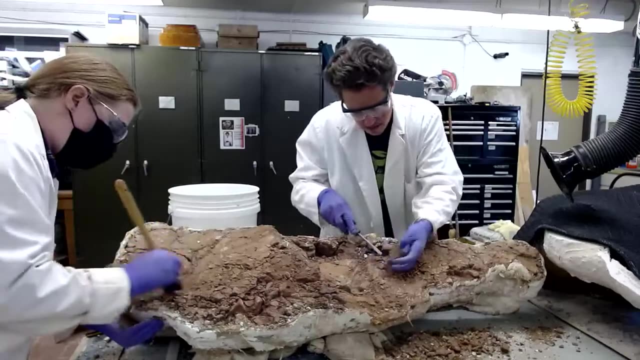 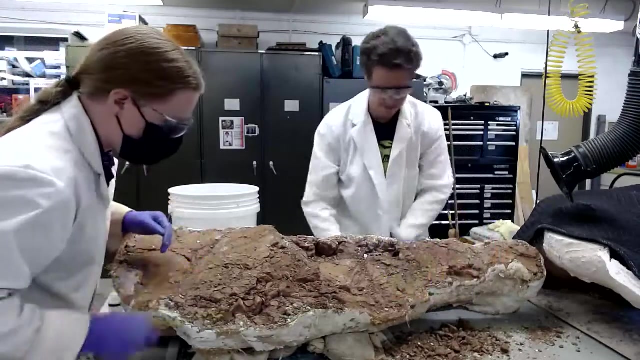 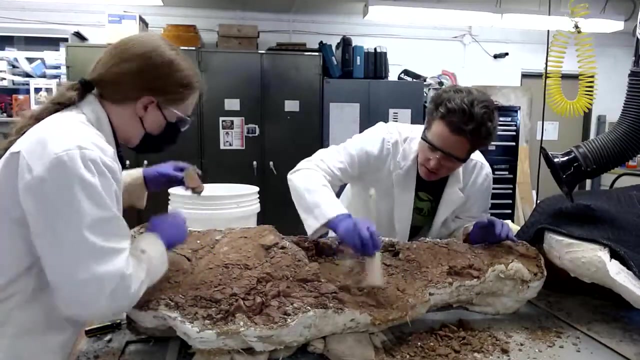 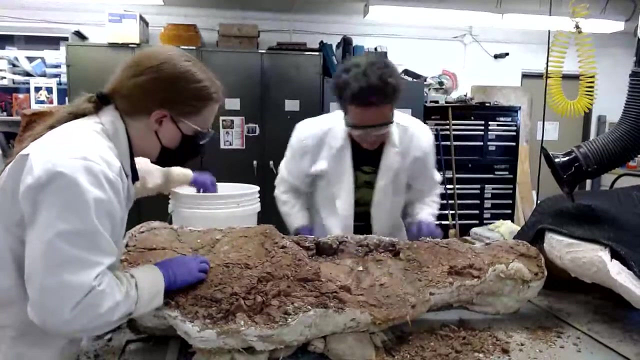 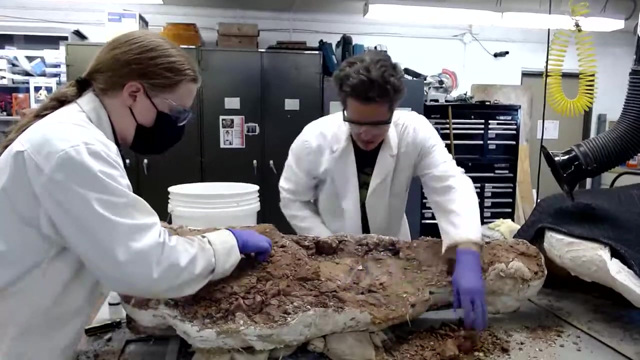 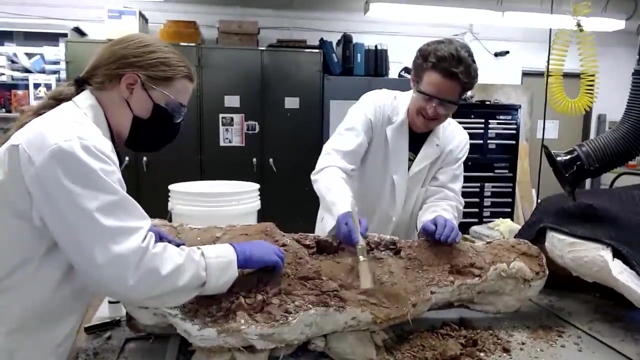 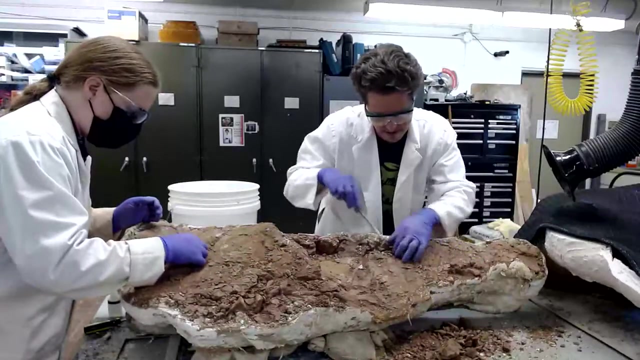 you never really know until you open up the jacket, kind of why this is christmas for paleontologists. Yeah, with prep, you never want to force anything. Could you tell us a little bit more about what Texas was like whenever this fossil- whatever it may be- was alive? 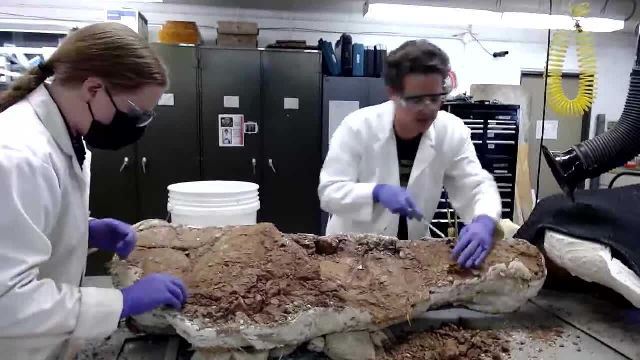 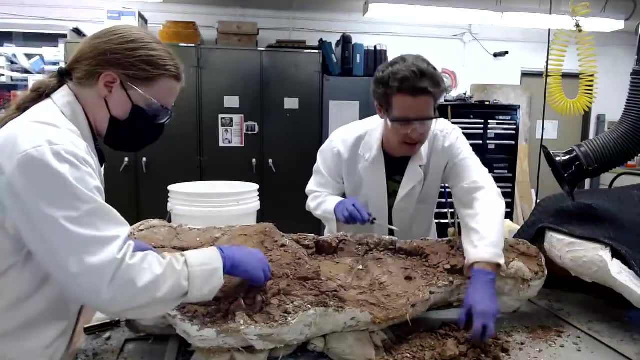 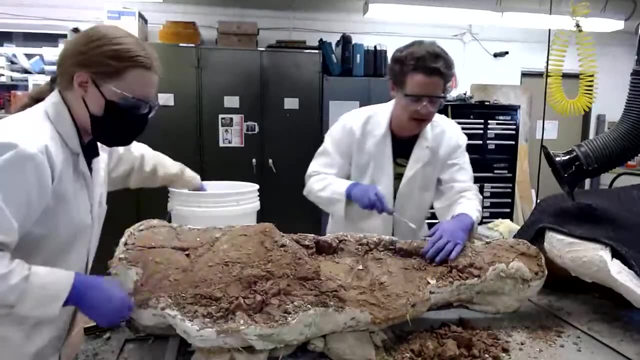 So, at least in the part of Texas where this was from, this animal would probably have been living in a broad, swampy plain, kind of similar to what you would expect in East Texas today: Low-lying areas with big meandering rivers moving towards the ocean. 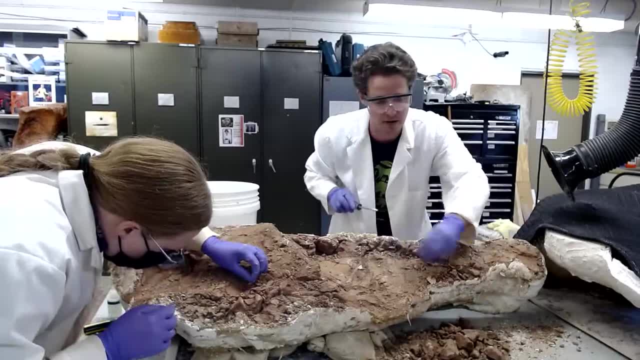 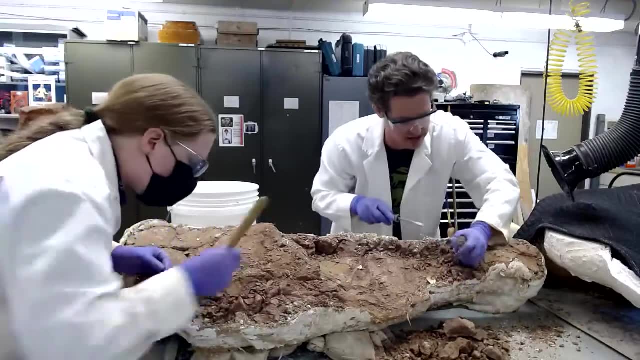 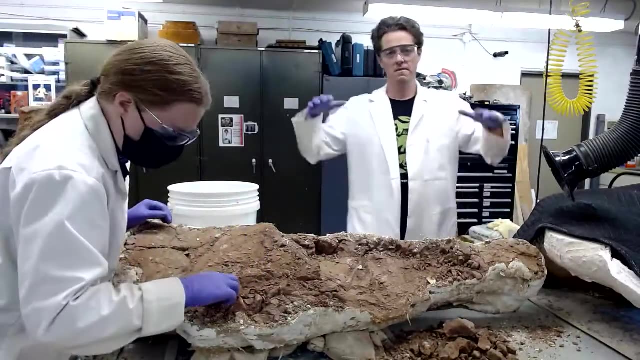 But in this case the ocean probably would have been directed more to the west, toward where We think of New Mexico and Arizona to be today, And this is Triassic. so at this period, Pangea, all the continents, have combined into one land mass. 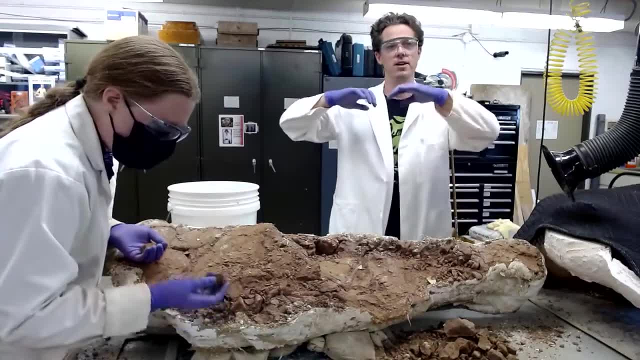 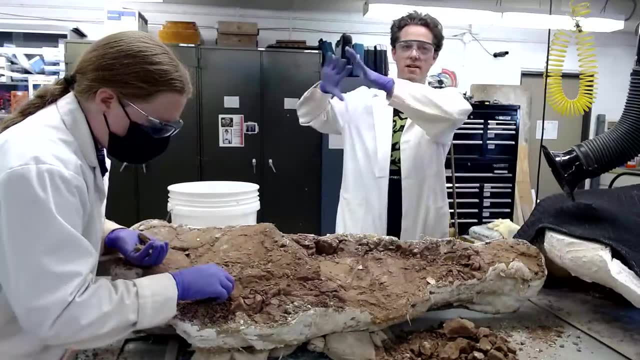 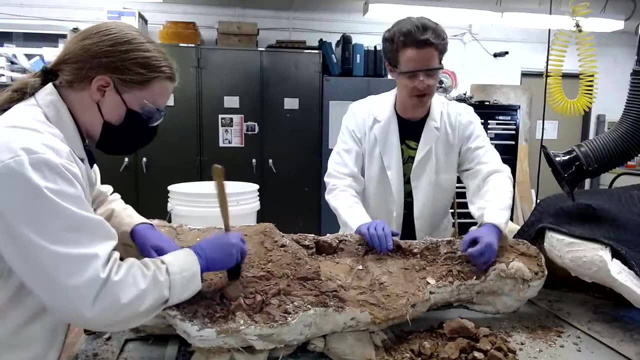 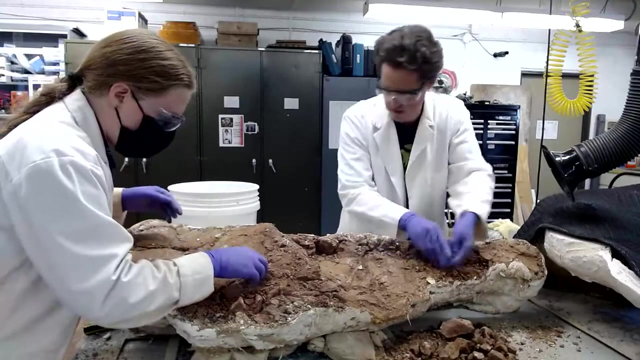 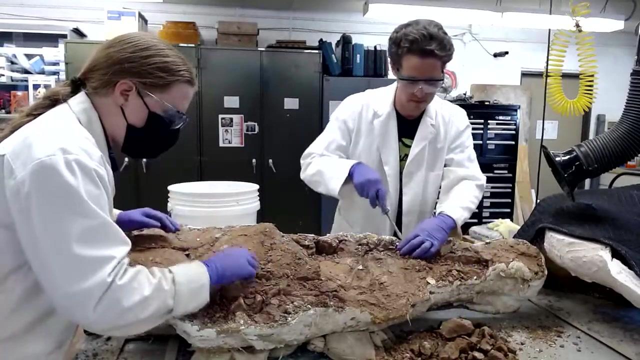 And it's just starting to break apart, And one of those openings probably would be toward where we have the gulf today, That would be the separation of either well, South America or Africa away from the southern United States. Is the age of the locality Norian. 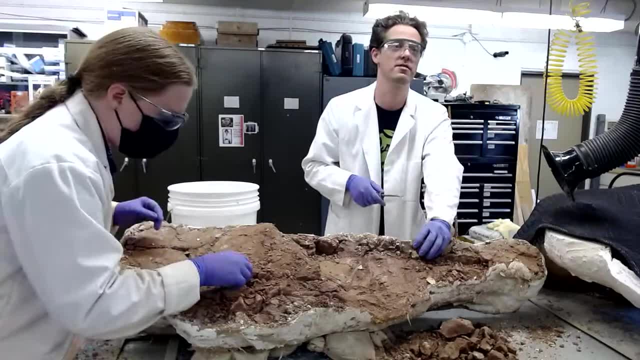 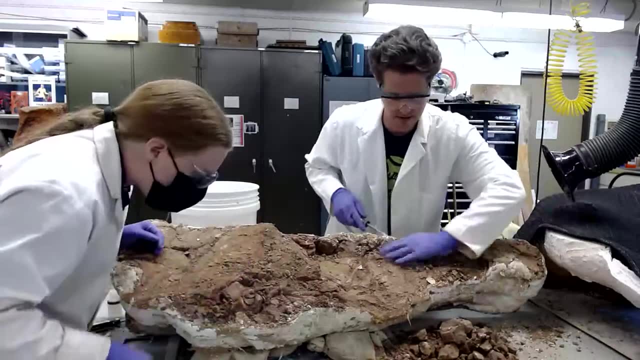 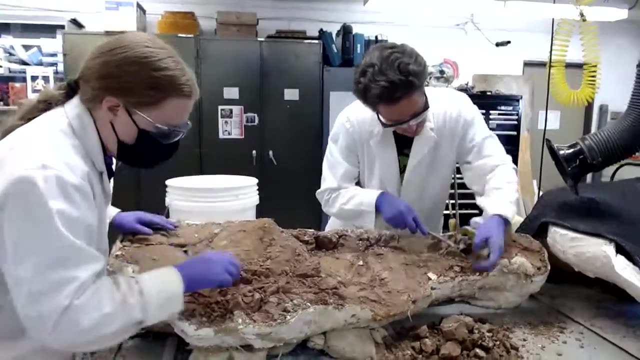 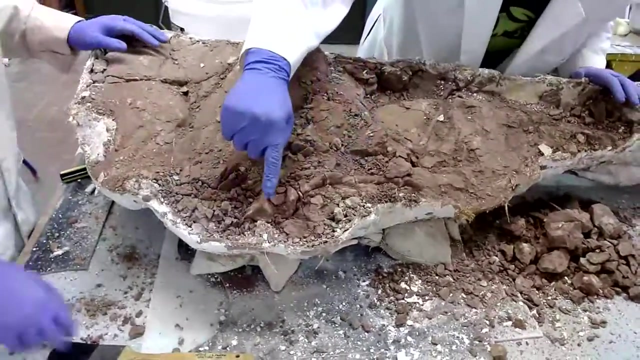 I would have to check to see if it is Norian age or Carnian. I would have to look that up to check. We would have to go back a little bit, Okay, So now we've got, we have our joint here and the bone that runs in this direction. 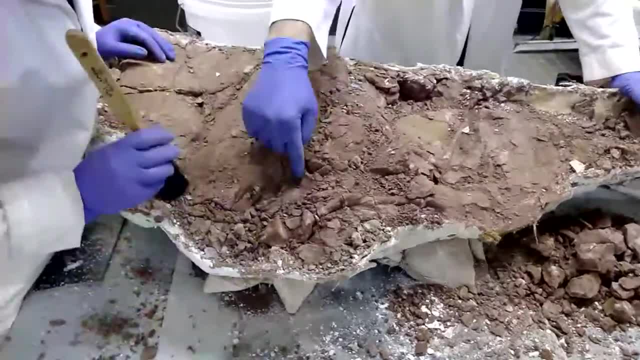 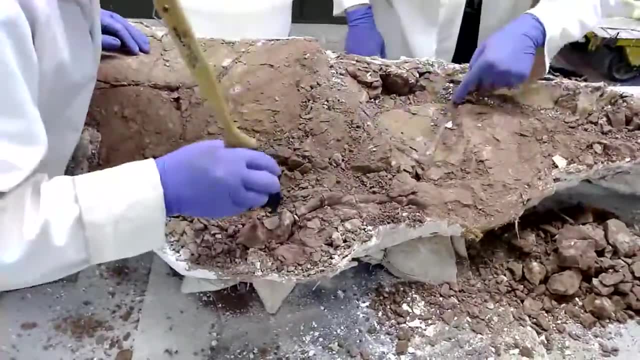 Then there is something else coming this way, So that is most likely the back or the underside of a Phytosaur skull, And probably what we have here is what's called a Gastrocancer, is what's called a gastralia, which is one of the ribs. 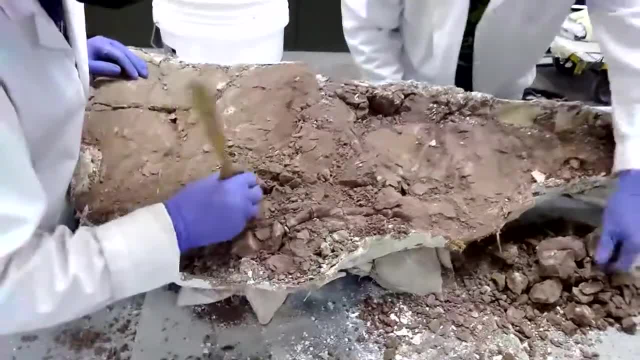 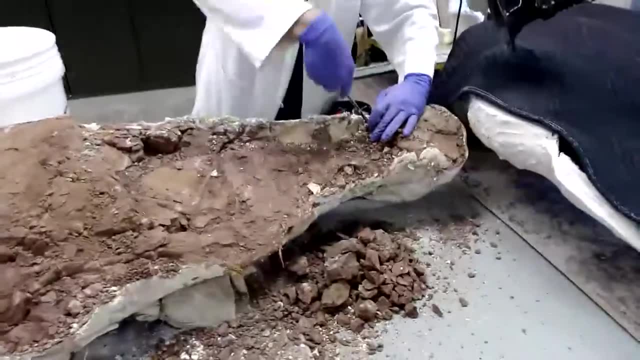 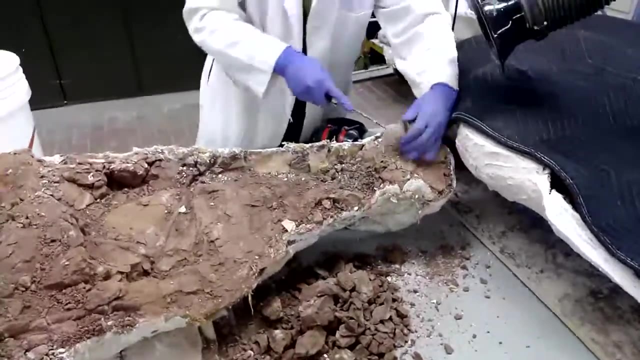 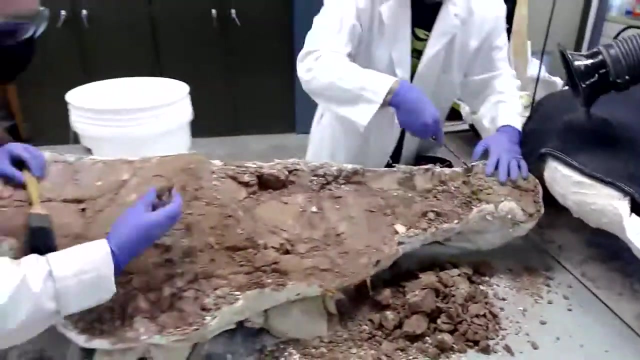 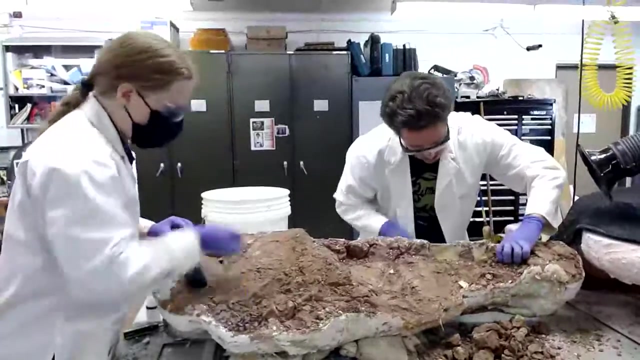 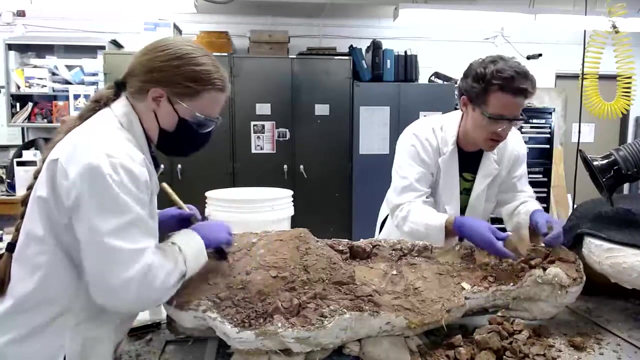 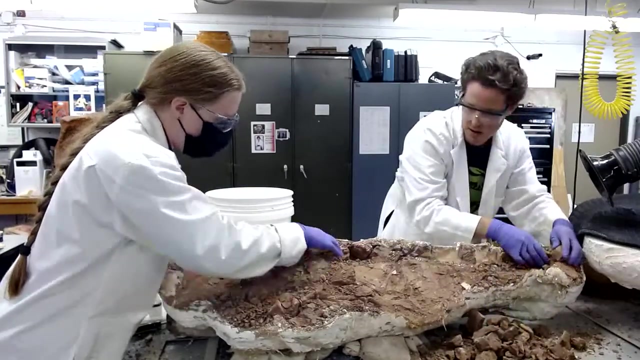 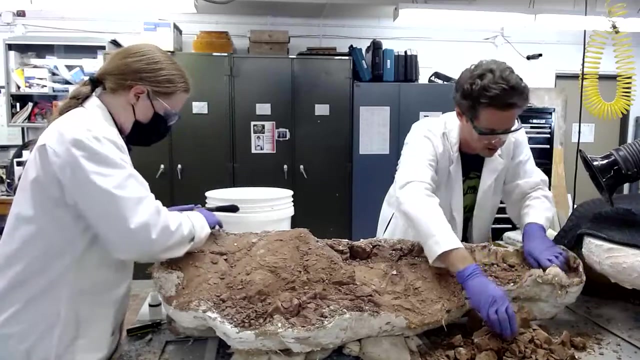 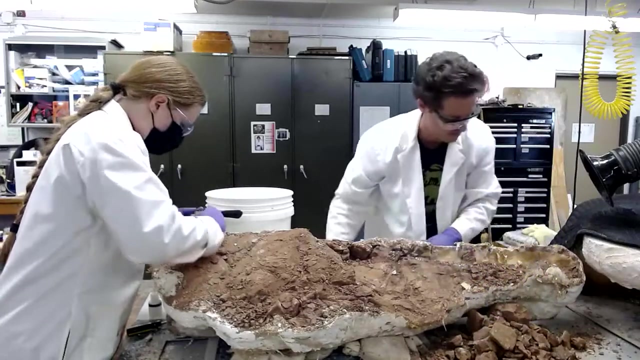 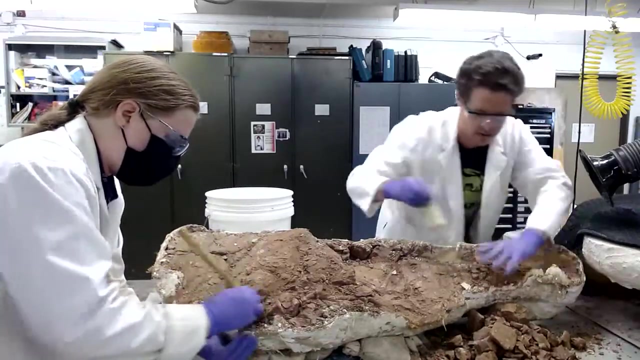 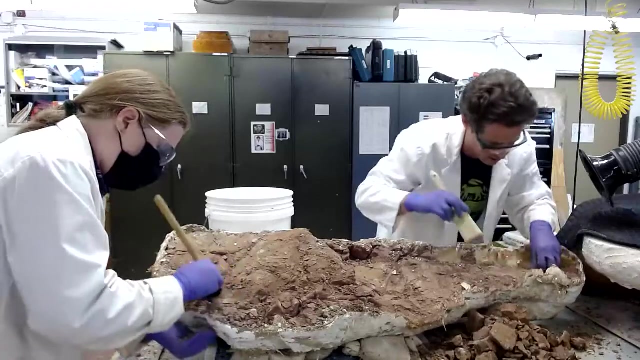 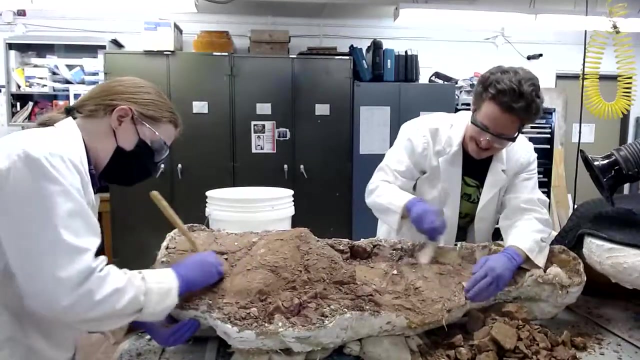 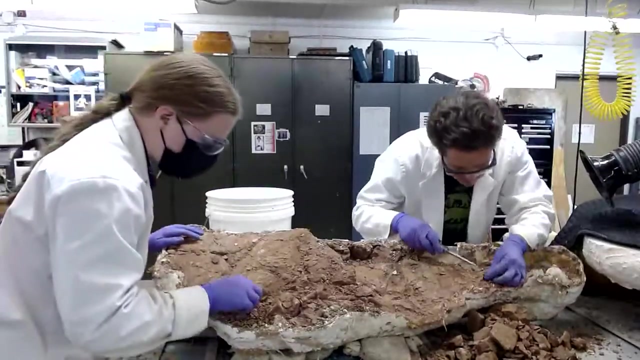 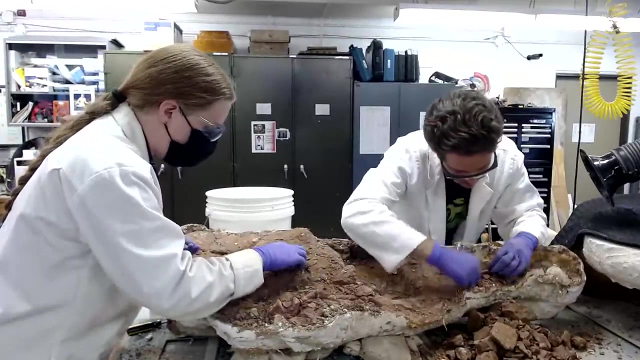 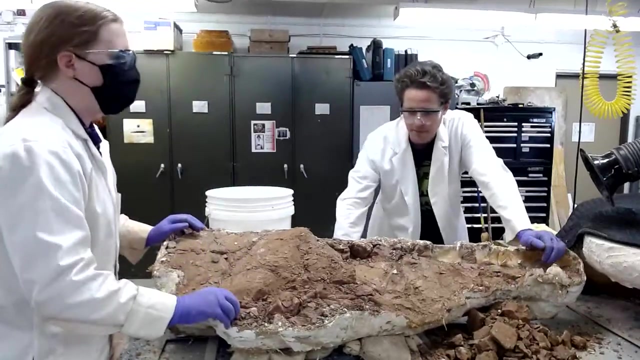 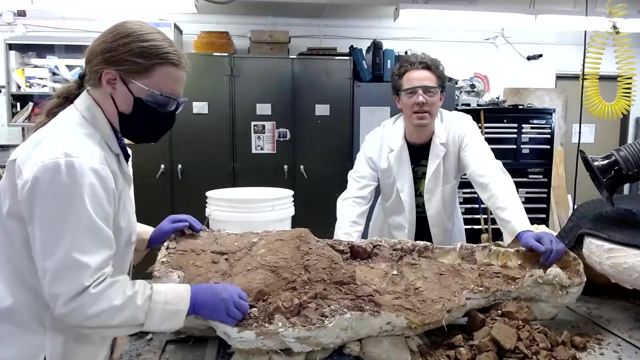 from the belly of the animal. All right, Here's something quiet and meditative about doing fossil prep. All fossils come apart this easily, or do you have to employ different methods sometimes? Sometimes we get specimens that are basically in a big concretion, a big hunk of limestone. 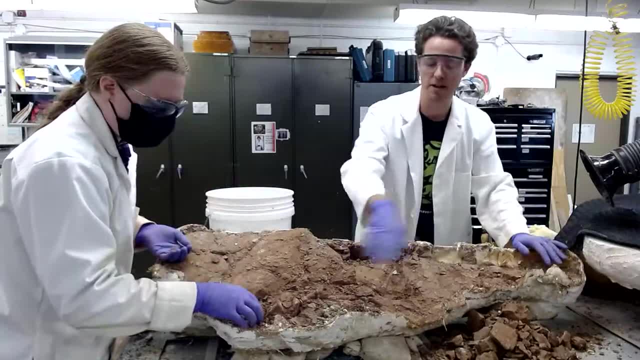 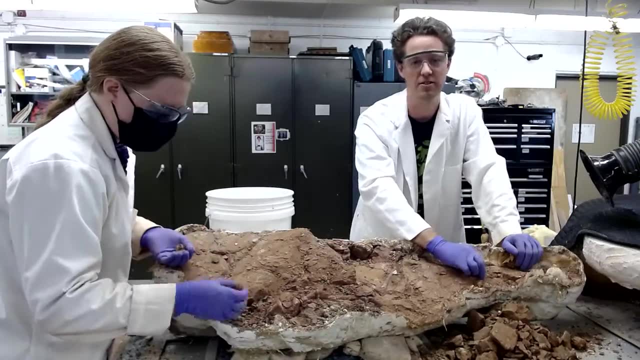 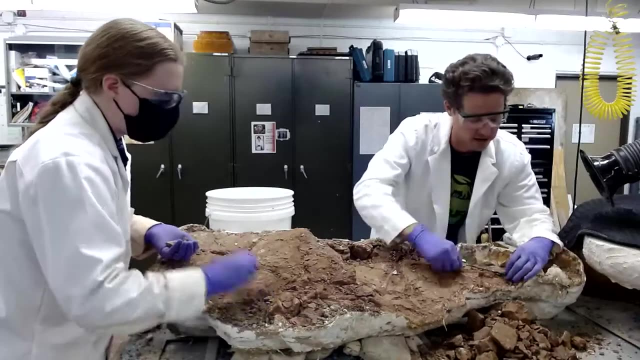 and the matrix around it doesn't crumble away and separate from the bone nicely. So we just have to sit down with a lot of our heavier-duty equipment like air scribes and slowly chip away the layers of bone, Or in some cases we might use acid to prepare away the rock. 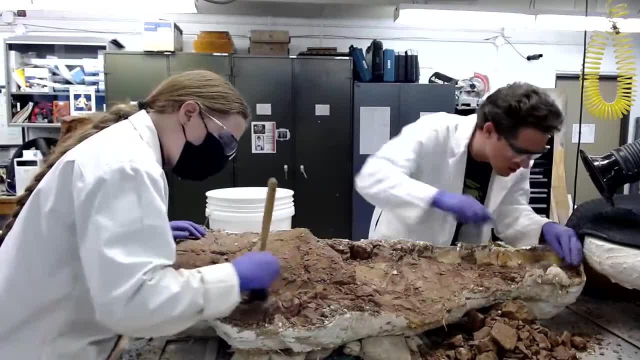 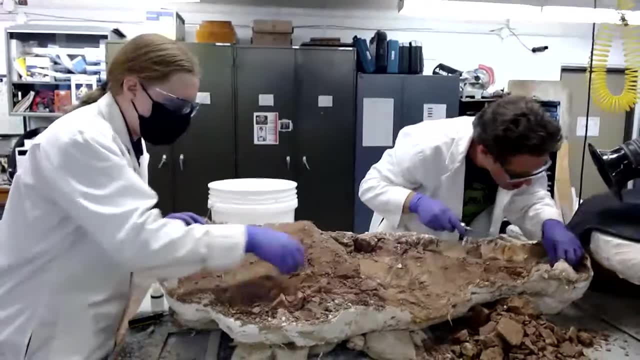 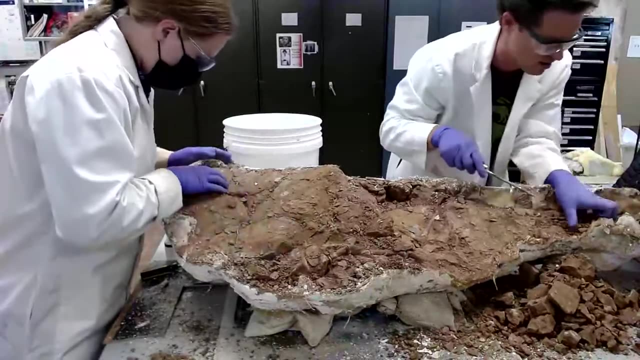 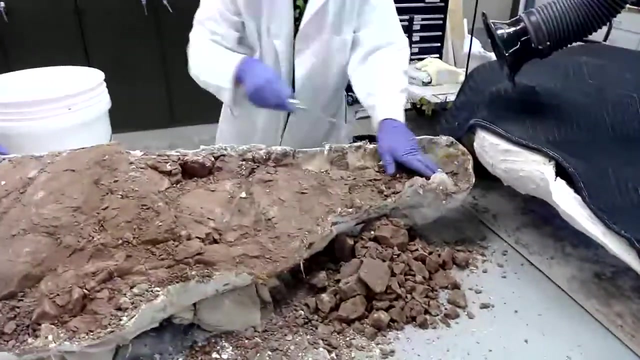 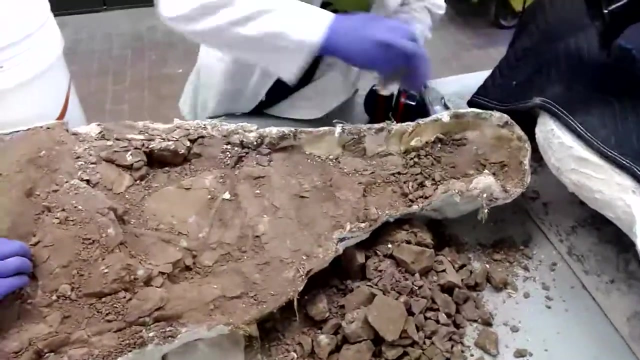 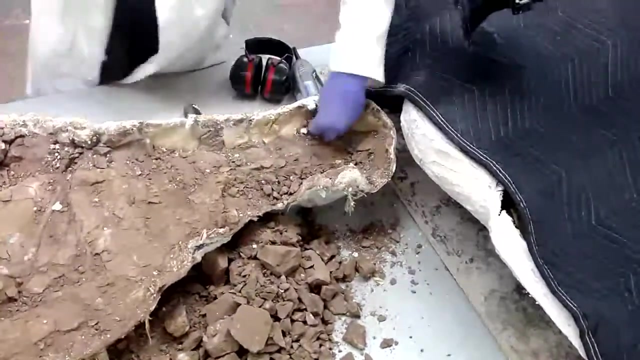 Hmm, I'm going to be able to choose. No, I started to think I had something up here, and if there is something, it's a lot deeper in the jacket. Wait, What have we got here? There we go, Yeah. 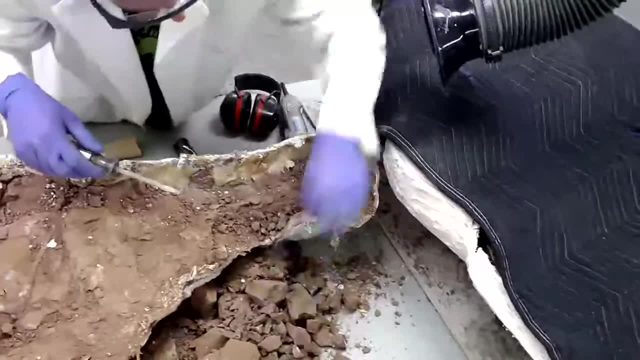 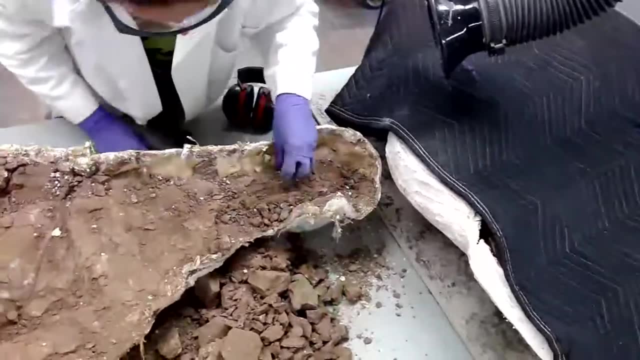 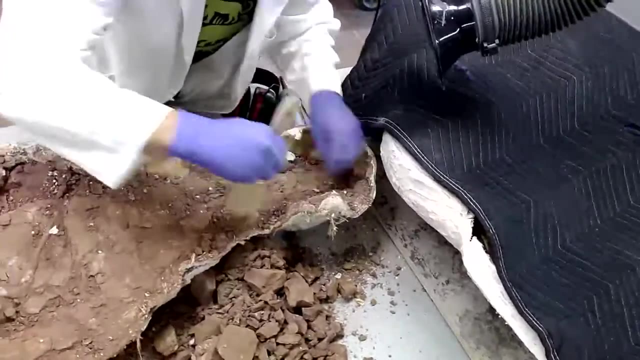 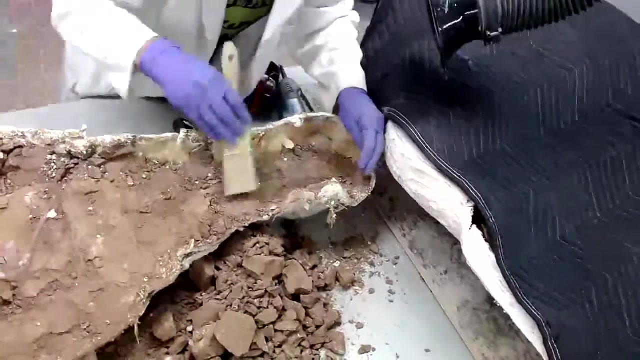 信用 … Perfect, Thank you so much. And there we go. We are pretty All right. So in this class, when we learned this technique, I didn't want to spend so much time with stimulus problems in theoretical recoveries any way. 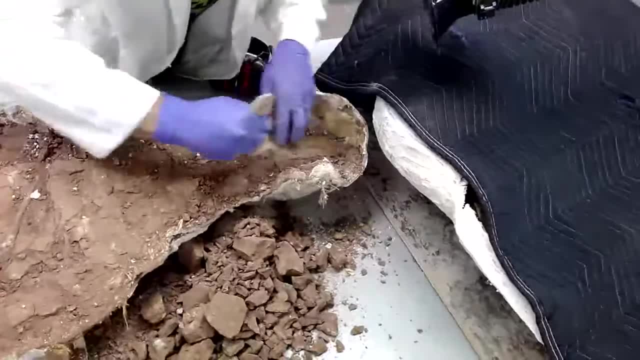 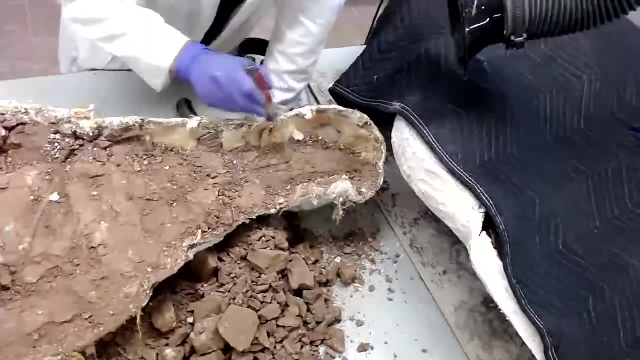 We didn't want it to be less satisfying, We don't want to spend time playing with blocks and we also don't want to go too far into class. Okay, so I've exposed more bone up here, and there's one bone running here. one running. 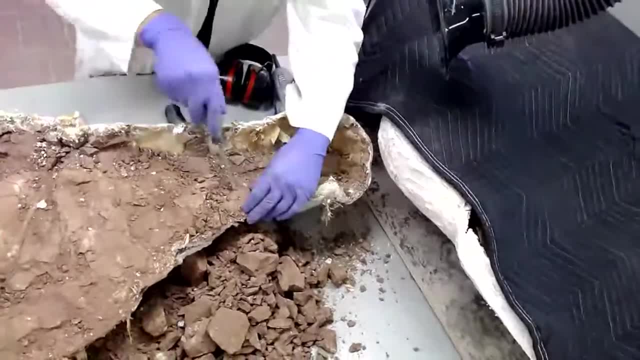 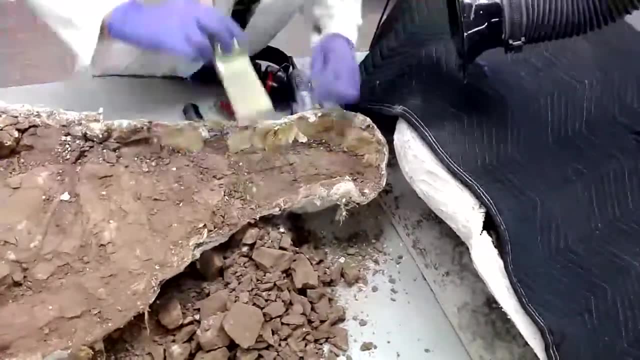 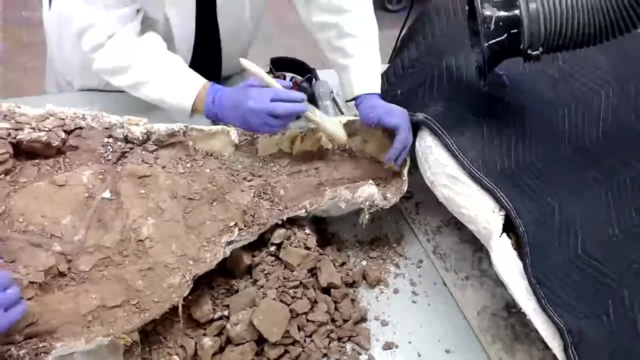 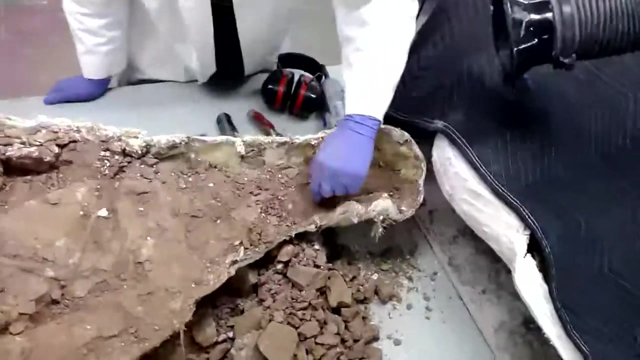 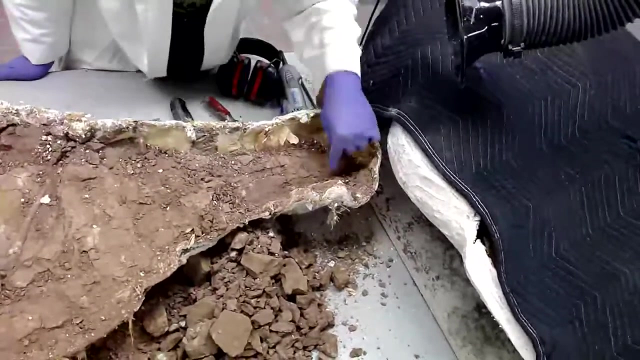 along here. It's not the most visible thing, but this is part of the jaw of the animal, So this is a phytosaur jaw, And what I've now realized that we're looking at is there are two bones that are running and splitting apart here and there is a little groove that has some spots that would normally 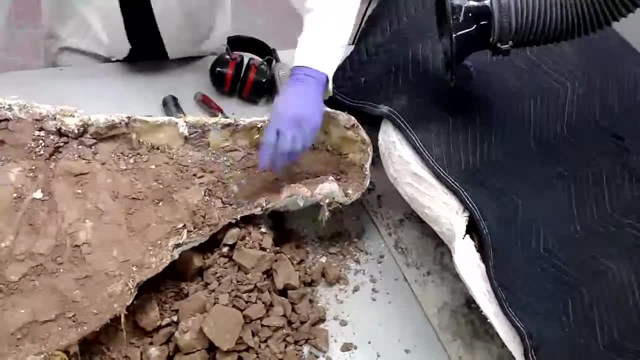 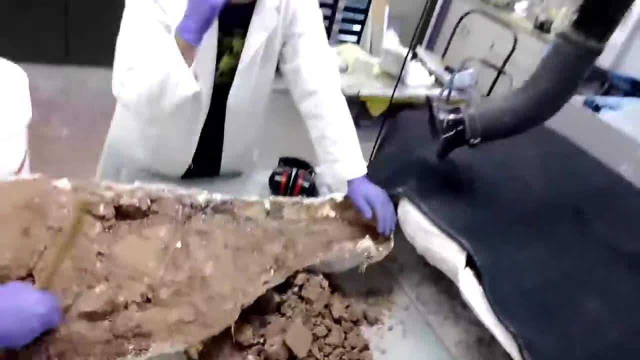 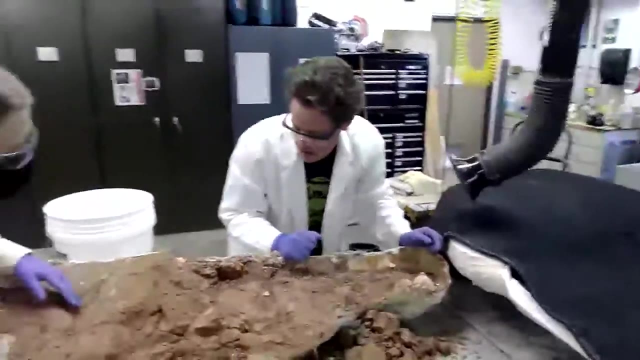 hold teeth. I don't see any teeth, And this bone probably runs out over here, So this is actually, instead of a skull, we're actually looking at the lower jaw of the animal. Okay, So it's a large phytosaur. 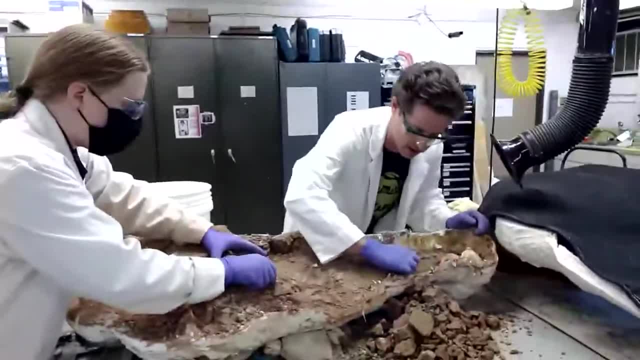 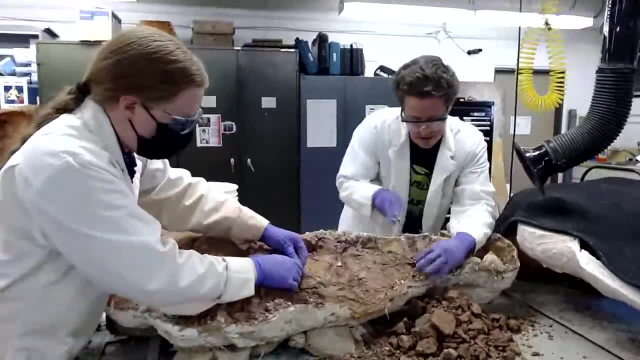 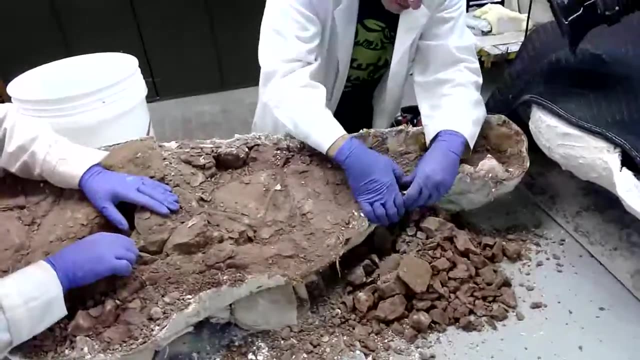 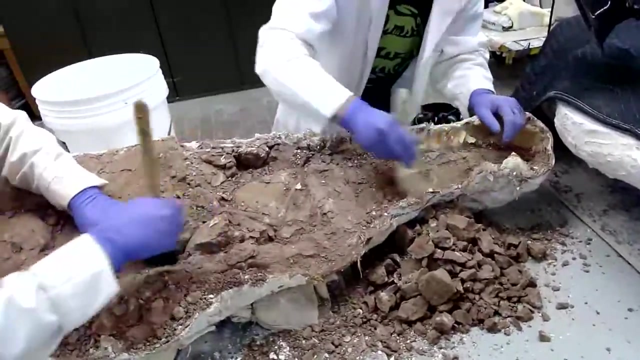 Let's see if I can clean up and follow that one bone all the way over. Okay, So this is the lower jaw of the animal And this is the lower jaw of the animal. And this is the lower jaw of the animal And this is the lower jaw of the animal. 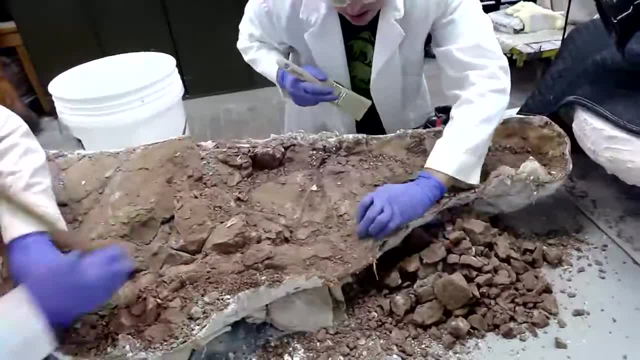 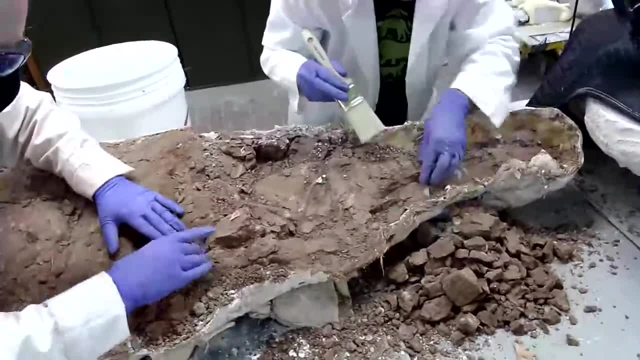 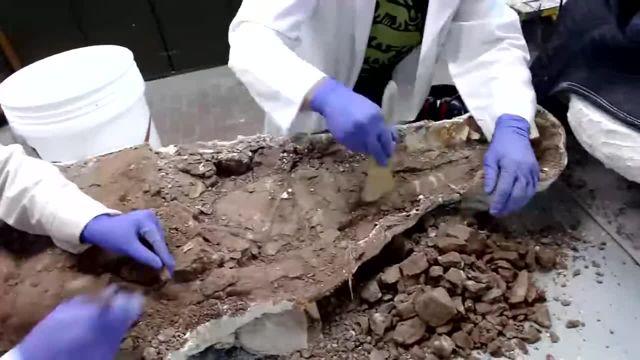 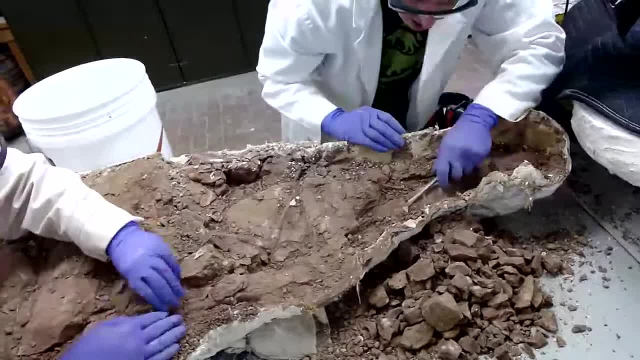 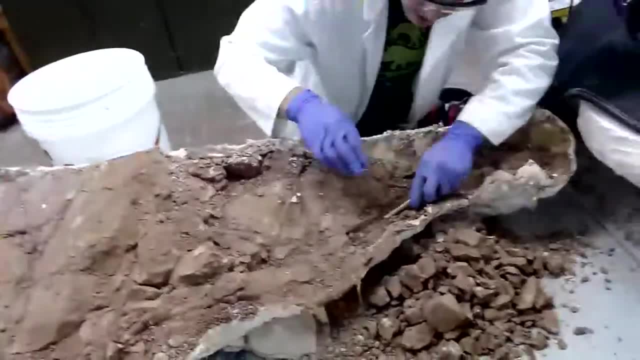 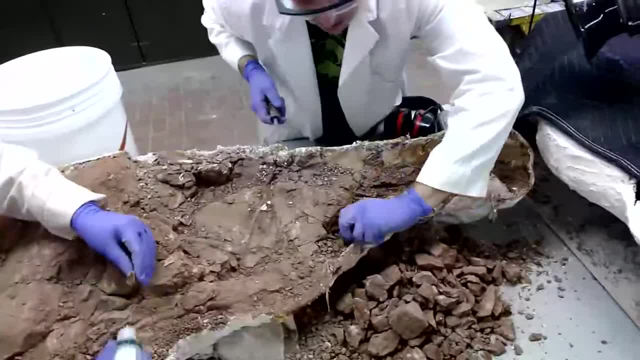 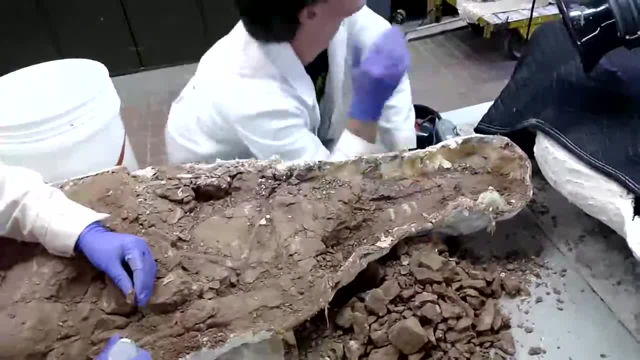 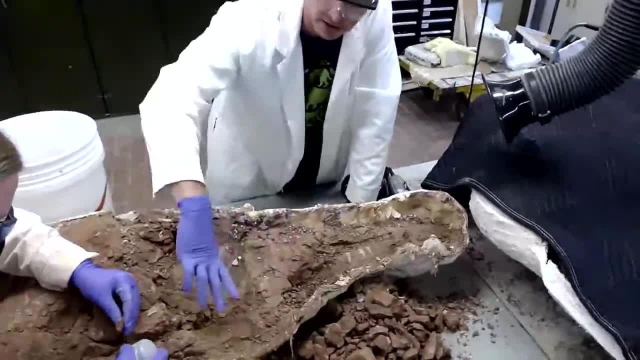 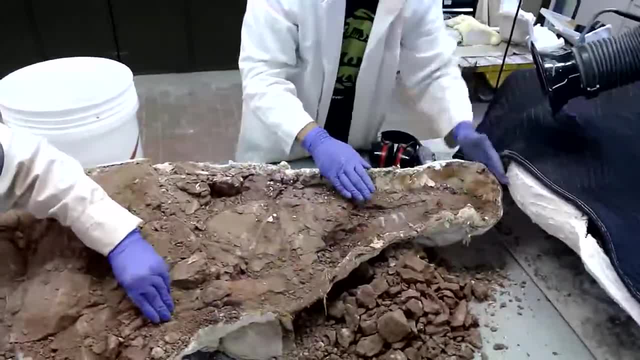 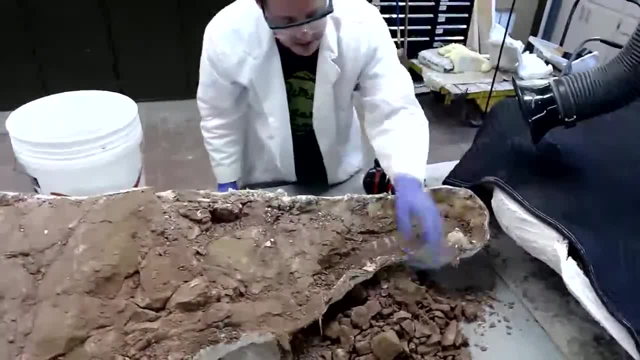 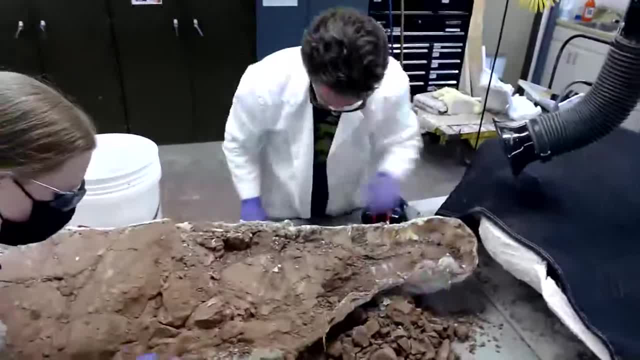 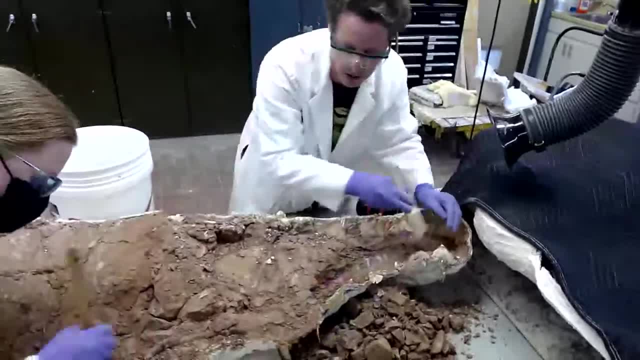 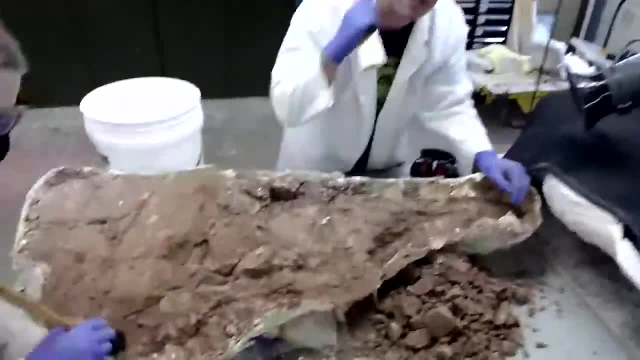 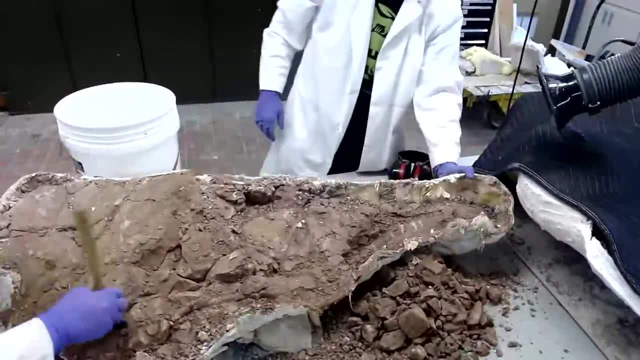 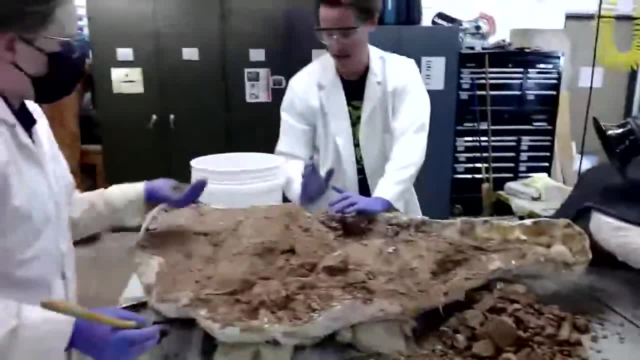 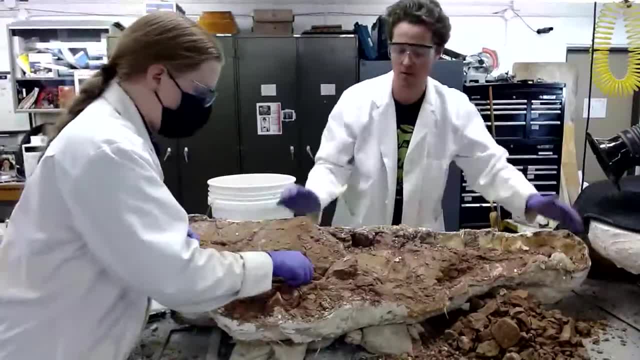 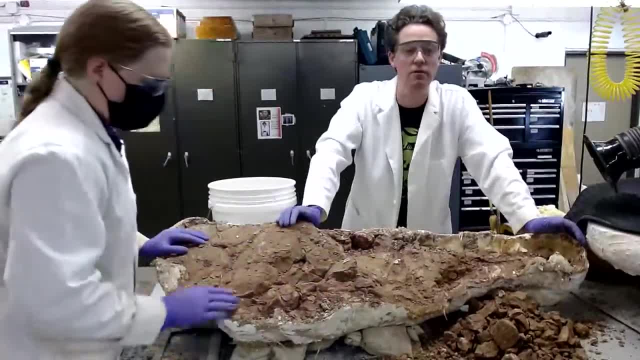 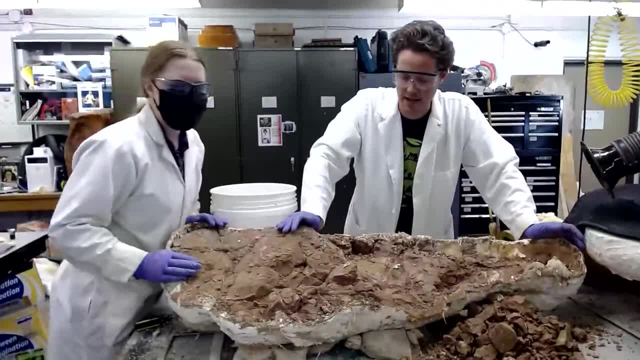 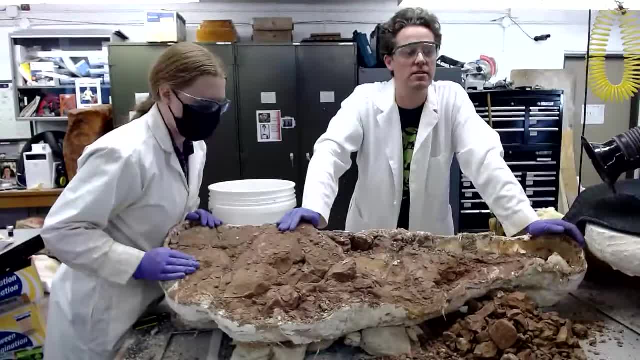 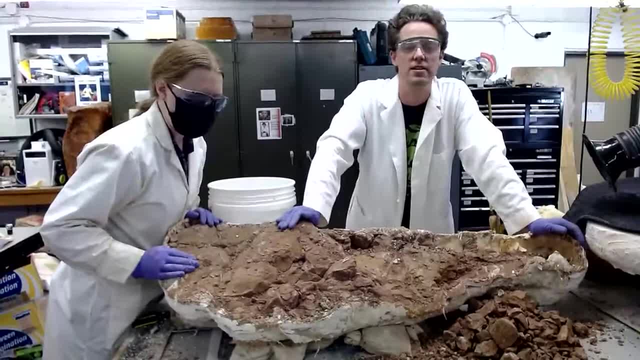 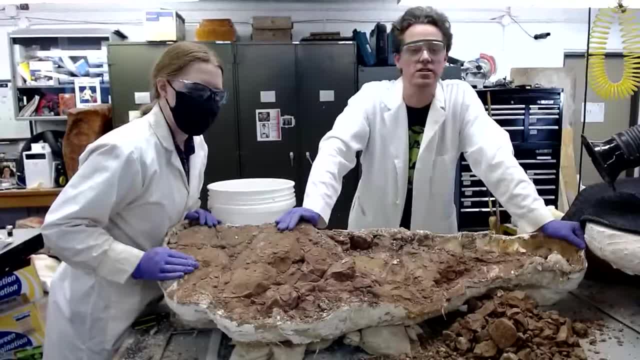 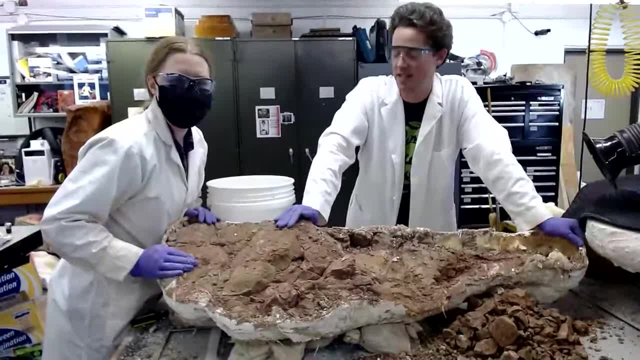 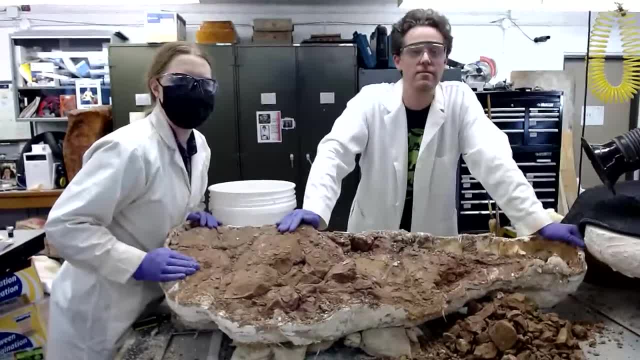 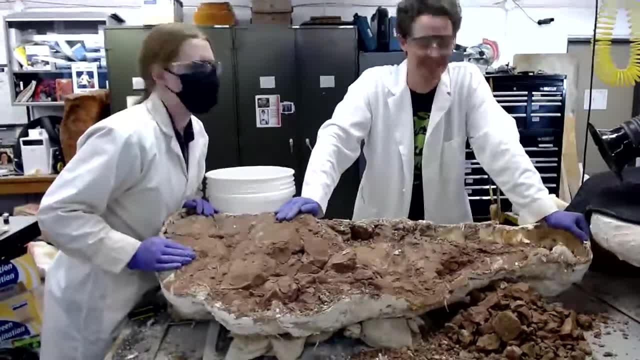 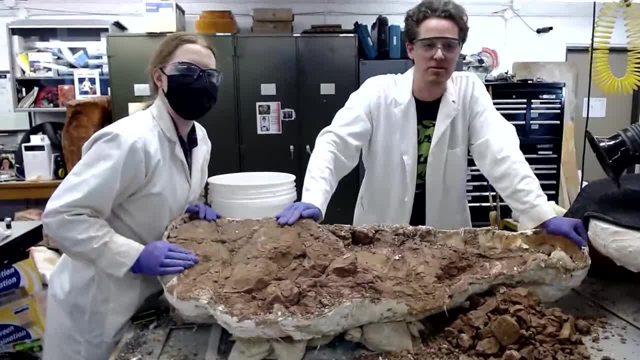 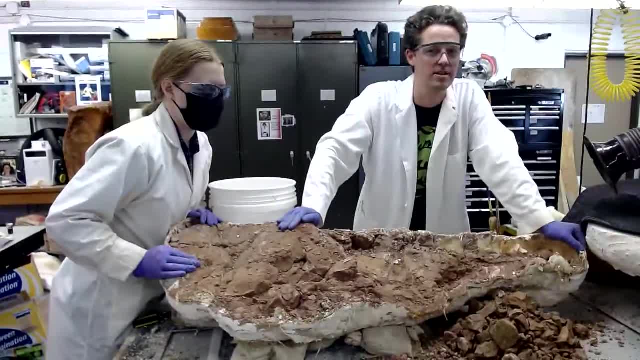 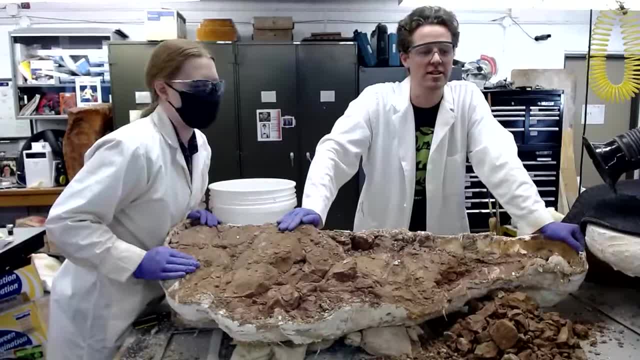 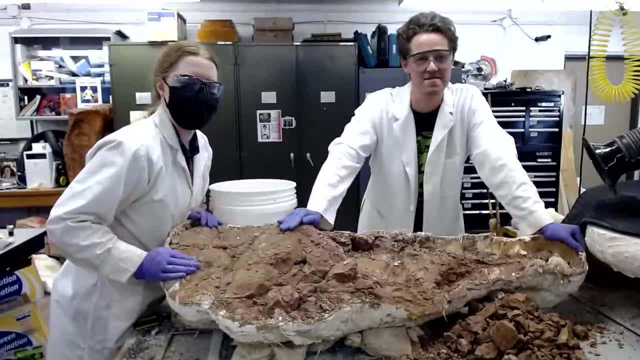 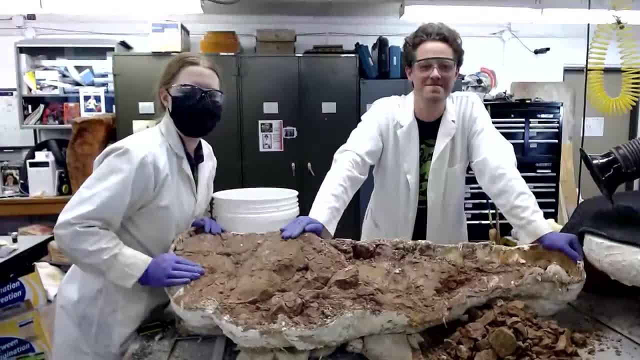